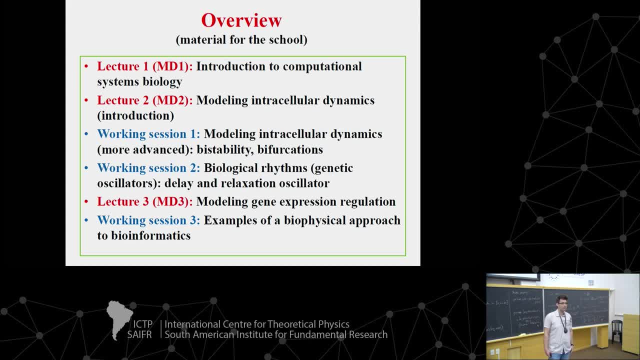 it by CRISPR-Cas9.. And this is this sort of very new and very hot topic in biotechnology. Basic idea is that it can edit any sequence in the genome that you want, So it can be used for basic biology and potentially it might be used for medical purposes as well, And there are. 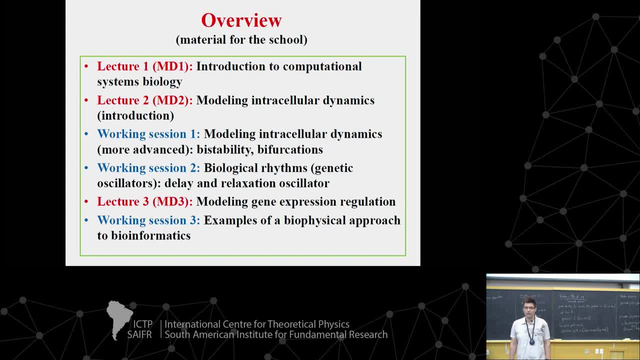 a number of controversies related with CRISPR-Cas as well, For example, designer babies, ethical issues and so on. 0. This is what we are doing, although we are not really focusing on this: biotechnological applications of CRISPR-Cas, at least not directly. 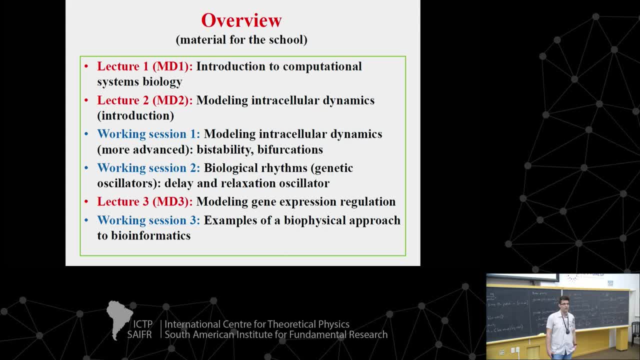 What we are trying to understand is how this system is natively working in the cell And then also by doing this you can make better ways to sort of use system in biotechnology and medicine. So this will be the lecture two and it will be really introduction. 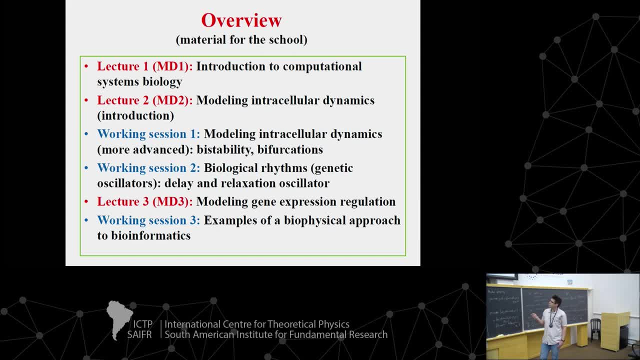 And now working session number one will also be on modeling intercellular dynamics, but it will be more advanced. So what we will cover is sort of basics of nonlinear dynamics Here, in particular bistability, bistable switches. We will also talk about bifurcations. 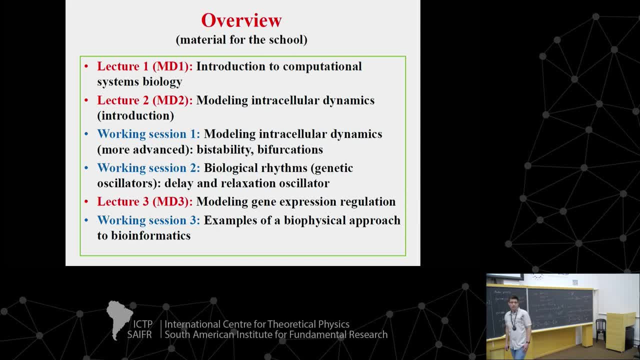 So in the lecture, the example that I will give you- actually there will be two examples- will be when you have just one stationary state, Which means system, The system goes from, say, zero to the stationary state And what is important is this: kinetics, how the system makes transition to the stationary. 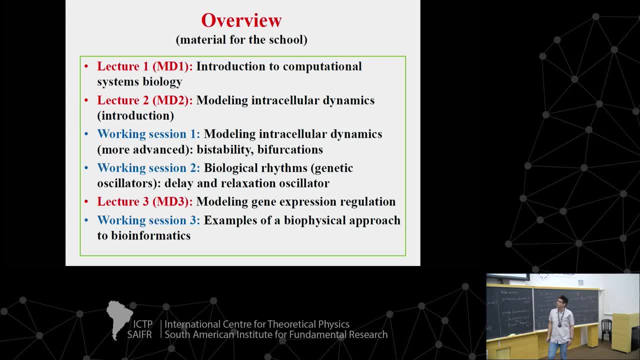 state. Now you can have, of course, more complex cases. For example, you could have two stationary states. then this is bistability And, importantly, topology of the stationary state can change, For example when you change the system parameters. 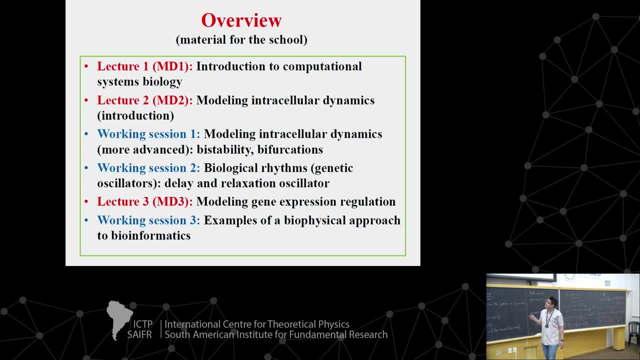 And this is bifurcations, So this will be covered under this work in session one, And then work in session two will be about biological oscillators, or genetic oscillators, however you want to call them, And the reason why Fernando mentioned that for work in session two you have to be on. 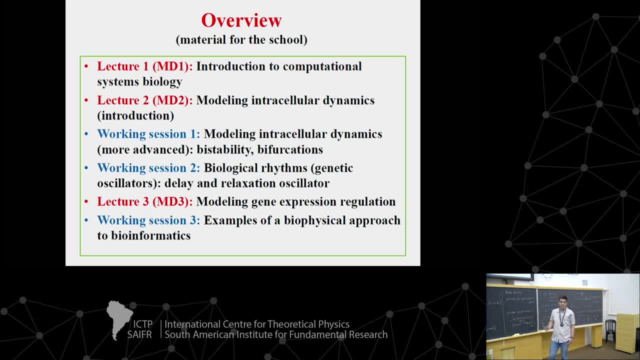 the work in session one is because bifurcations are really needed in order to understand, at least quantitatively, how oscillators are working. So this is why these two work in sessions are interrelated with each other. Thank you, Thank you. 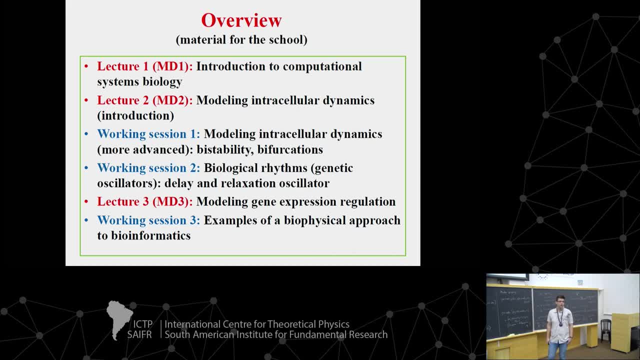 You have to be able to understand how oscillators work and how they collide with each other, Although, for example, if you think that you know enough of the nonlinear dynamics, you can come, as far as I'm concerned, only to the work in session two. 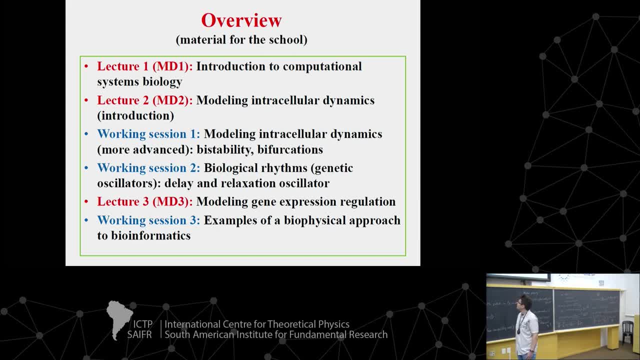 Now lecture number three will be about modeling gene expression regulation. So regulation is really the key issue in systems biology. So up to now, what you have heard is many interesting things about- mainly about single biological molecules. For example, many interesting properties of proteins. 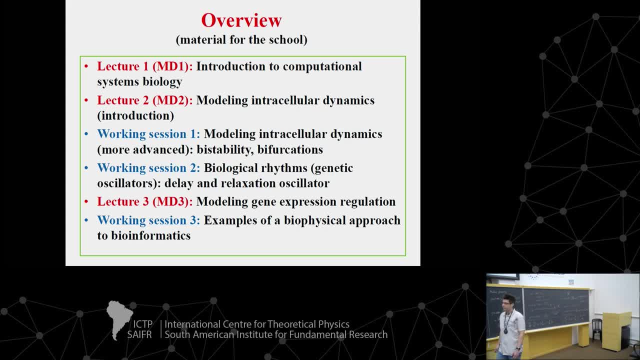 But then what is really important for systems biology is to understand how, first of all, these molecules- different molecules- come together- For example, proteins, DNA, RNA- how they interact and how these interactions determine the property of the entire system. This is why it is called systems biology. 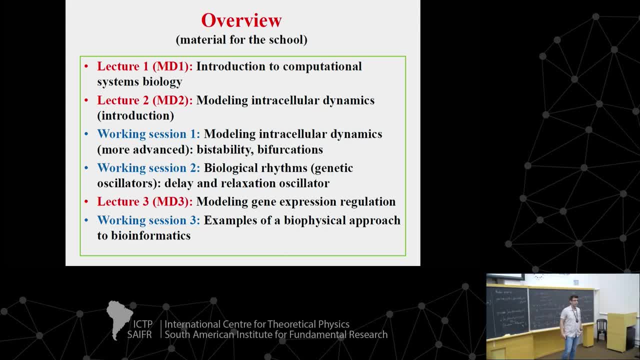 And also, by the way, this is why- because I mean, there are people with many different backgrounds here. So in this first lecture I will also give a brief introduction to basic molecular biology, essentially focusing on regulation and on DNA and RNA. 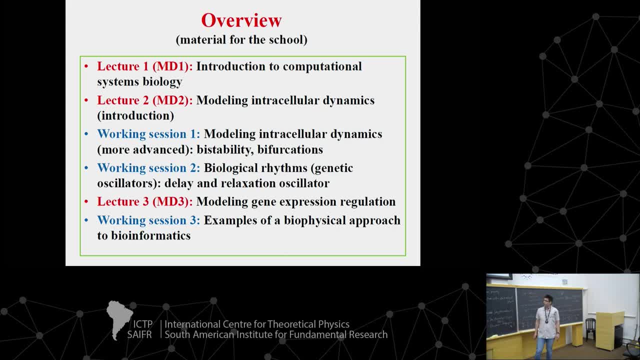 because you heard much about the proteins already. And then working session number three. it will be something different, So it will be on bioinformatics, which is actually tightly related with systems biology, But it will be bioinformatics from the perspective of biophysics. 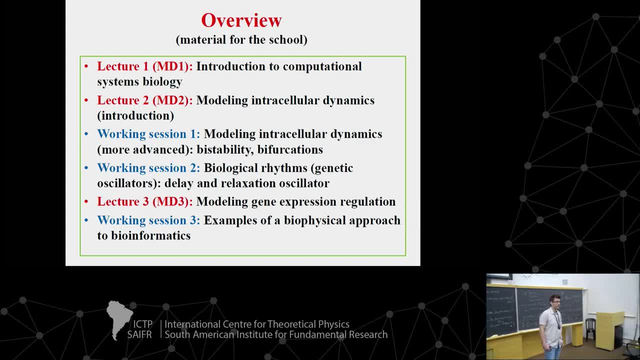 which means how we can use biophysical understanding of different systems in order to improve the ways in which we analyze biological data. So that will be the working session three. Okay, So this is sort of the overview, And then now is the overview of this. 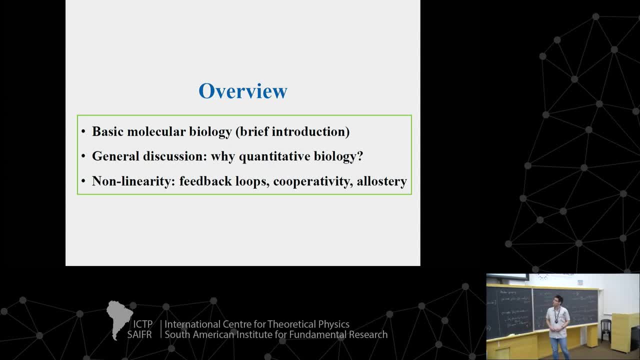 First lecture. so first I will be telling something about, as I mentioned, basic molecular biology. So the focus will really be on regulation, And as an example of regulation I will actually give regulation of transcription. So regulation of transcription is the most common point. 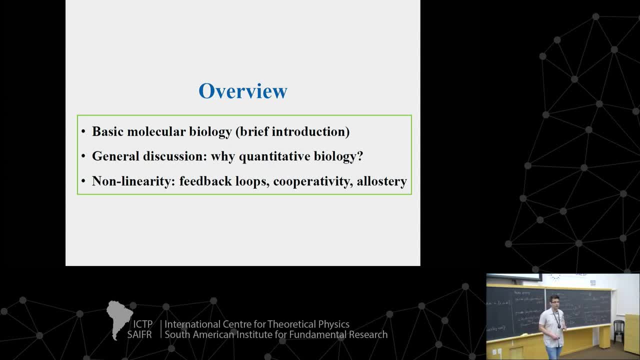 where the things are regulated when you go from DNA to the protein. Of course, as I will mention, you can have other types of regulation, but sort of as a model and as a focus, we will talk about regulation of transcription. Now we'll have sort of general discussion. 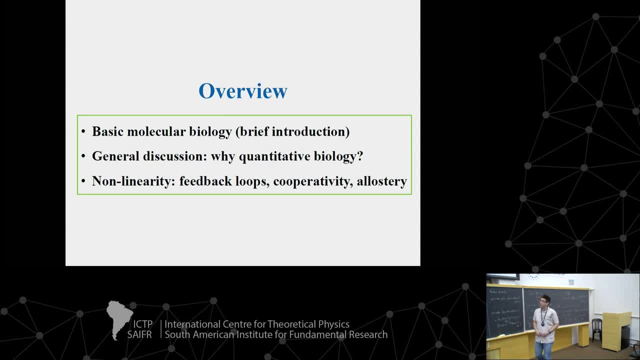 brief general discussion, because it is an introductory lecture, of why mathematical or quantitative modeling is needed in biology, And then the last part of the lecture will be about nonlinearity- why nonlinearity is very essential in biological systems And related with this. we'll talk about feedback loops. 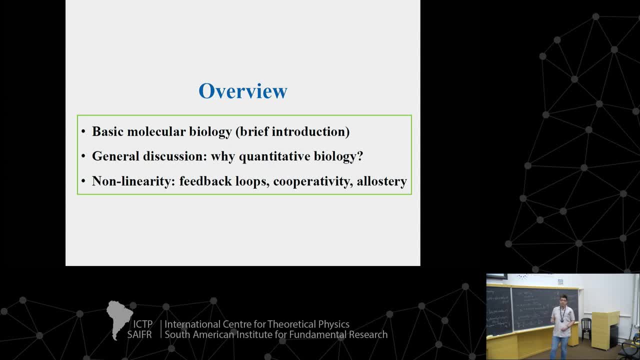 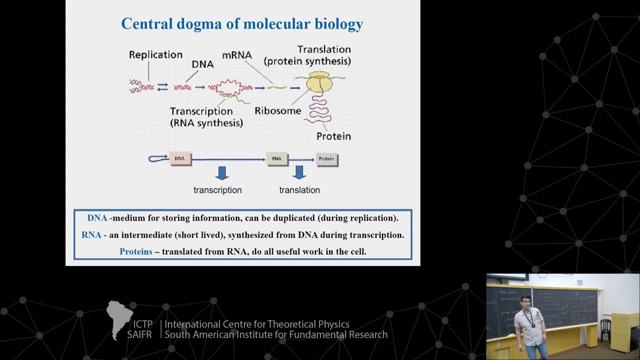 about cooperatives and about nonlinearity, to which this nonlinearity is very often achieved, And also about the loss tree which goes along with cooperativity, often. Okay, so here's the overview of basic molecular biology. Now you have already seen, I think, a few times. 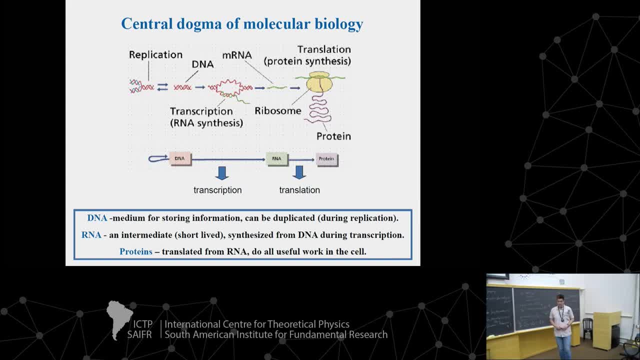 the central dogma of molecular biology, And actually I will mention the central dogma a few times during this first lecture. So what is the central dogma of molecular biology? So what central dogma really emphasizes is flow of information. So it says that information flows from DNA to RNA, to protein. 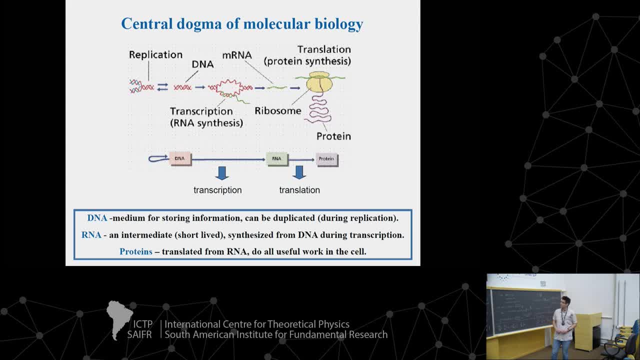 So, first of all, DNA can be duplicated in the process which is called replication, And when you think about DNA, it's a very stable molecule, so you can view it basically as a medium for storing information. Then we have transcription, which is a process in which RNA is synthesized from DNA. 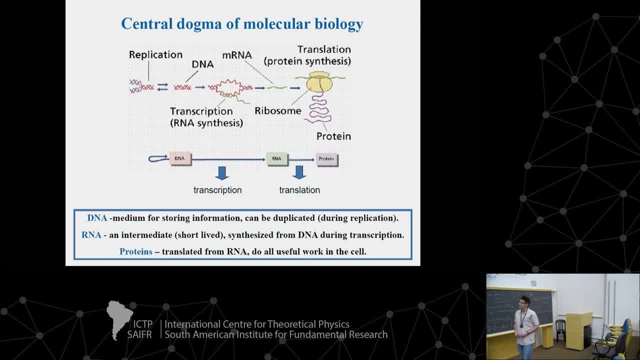 And RNA is sort of intermediate between DNA and proteins, although it can have many other very interesting functions as well. It is typically short-lived, so the half-life of proteins is on the order of minutes, as opposed to the proteins, which are typically very stable in the cell. 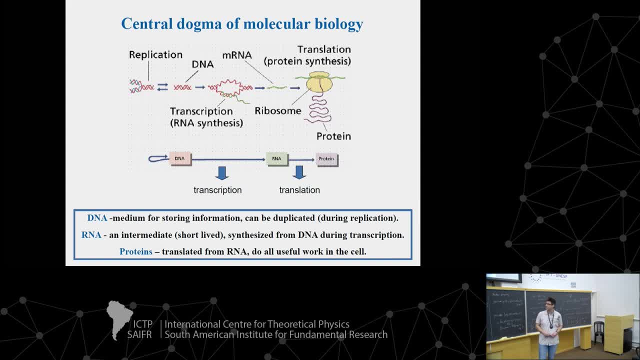 Their half-life is on the order of hours or even days. So once we have RNA, then protein is synthesized through the process called translation, And once we have proteins, proteins are actually doing most of the work in the cell. They can catalyze chemical reactions as enzymes. 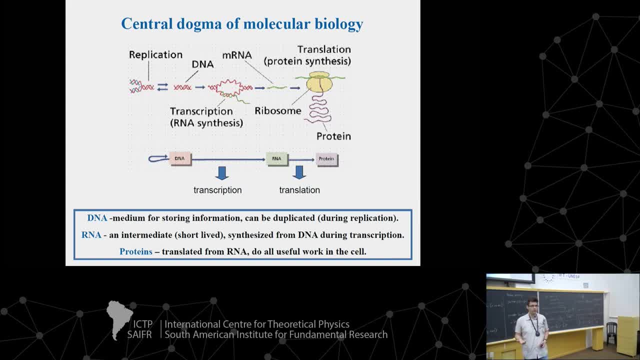 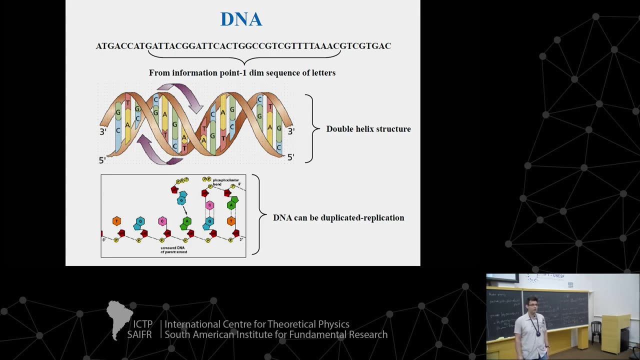 they can have structural properties, they can serve as molecular motors and so on. Okay, so this is the central dogma, and now we are starting from the first player, from the DNA. So, in sort of first approximation, you can view DNA as a one-dimensional 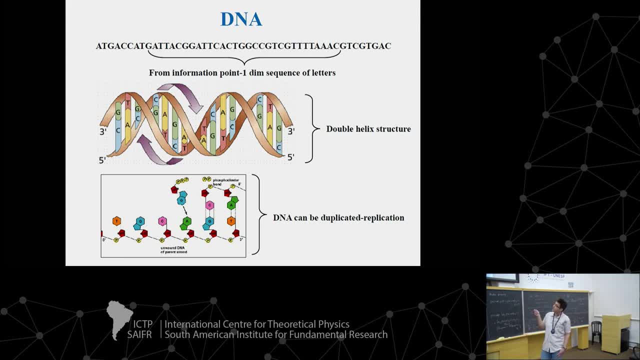 sequence of letters. So here you have a piece of DNA, and actually this simple representation is quite good for many purposes, For example for bioinformatics. let's say that you want to find some motifs in this DNA sequence, and so on. So all you need for this purpose is actually this 1D information. 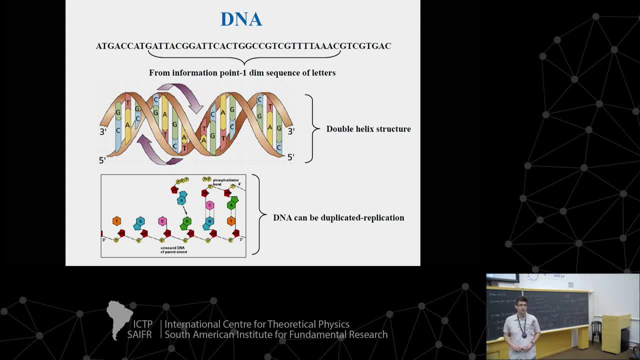 Now, of course, what we should keep in mind is that DNA has a structure, and this structure, of course, can be very important. For example, you may want to bend your DNA, you may want to twist your DNA. DNA can be also melted. 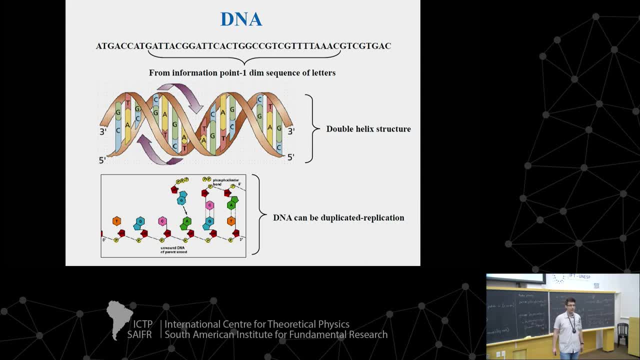 meaning that the two strands of DNA can be separated, and so on. And these processes can be very important as well. They can be important in modeling, they can be important in bioinformatics, and so on. Now I also mentioned replication. 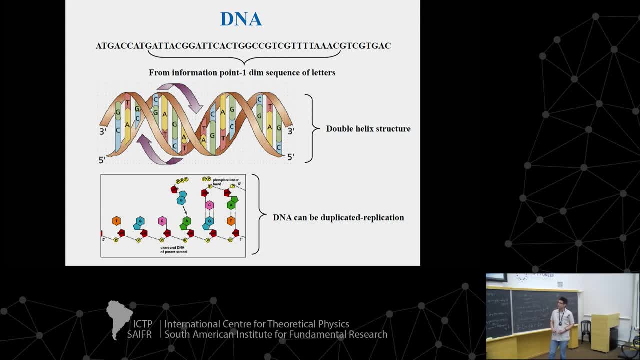 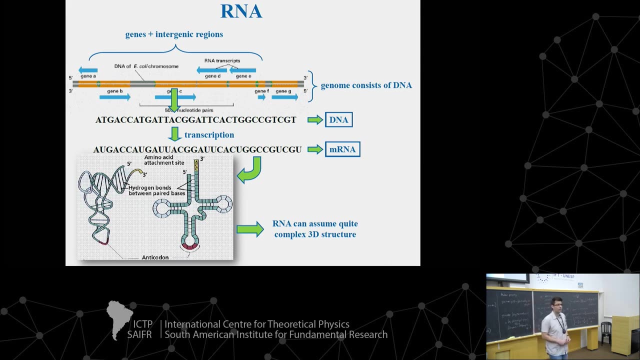 so what is just briefly shown here is that the replication works by having one of the two DNA strands as a template and using this template, you're synthesizing the other DNA strand. Now here, before going to transcription, I should briefly mention or explain what is the structure of genome. 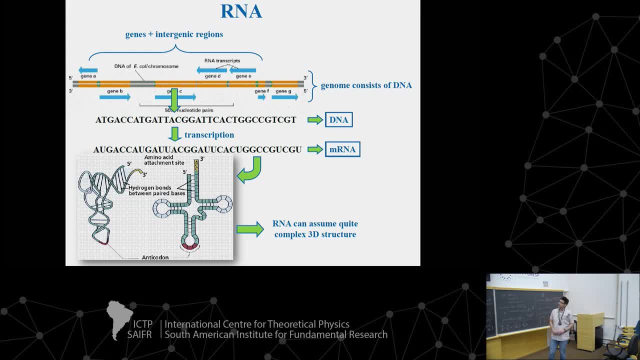 So here you have a piece of genome and then roughly genome can be divided to genes. so genes are shown in blue here and they can be divided in intergenic regions. So genes are pieces of DNA which code for proteins. So from gene you get your messenger RNA. 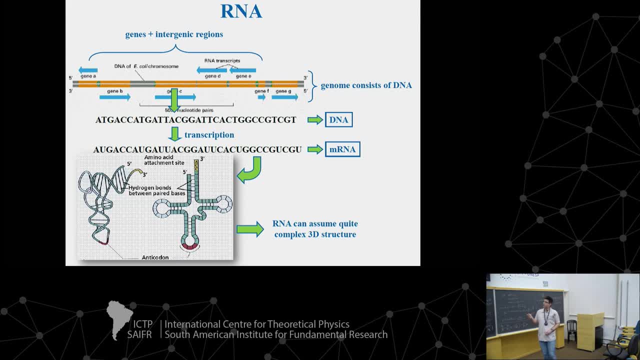 then from messenger RNA, you, by translation, get proteins And then these pieces of DNA in between. they are non-coding regions of DNA, they do not code for proteins, but they can actually have a very important role, And this role is mostly in regulation of transcription. 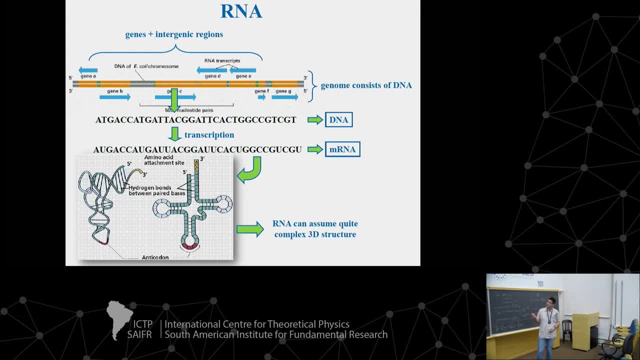 So you can have signals here which tell every gene when it should be turned on, when it should be transcribed, to what amount it should be transcribed and where it should be transcribed. So, for example, if you look at our cells, 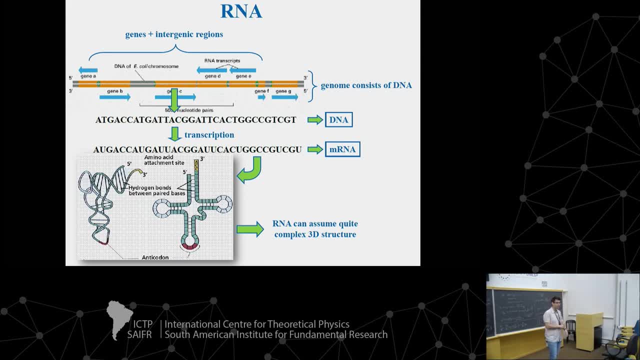 the cells in our body. if I look at my skin cell and, for example, at my brain cell, they are very different, obviously, but they have the same DNA And what actually distinguishes the brain cell from the skin cell, for example, or any other cell? 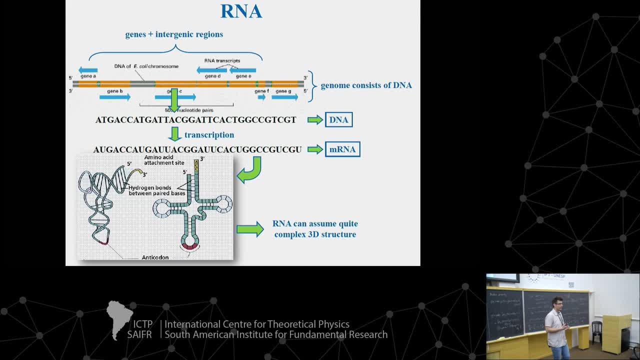 is actually regulation of gene expression. So different genes are turned on in these different cells, and this is actually determined by these short signals which are in these non-coding parts of DNA. So then, from gene, that is from coding parts of DNA. 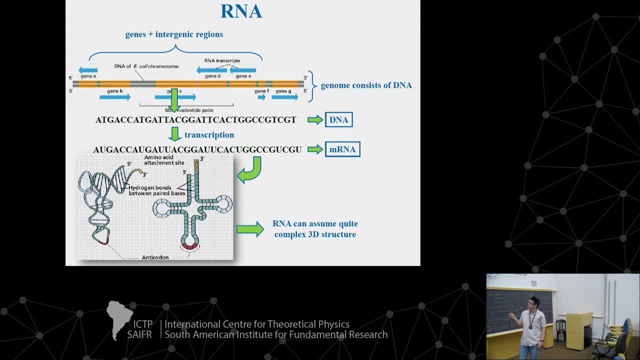 by the process of transcription we get messenger RNA And then messenger RNA gets folded And this is called secondary structure of messenger RNA. And this secondary structure is mostly what determines the properties of RNA. For example, if you want to see how your RNA 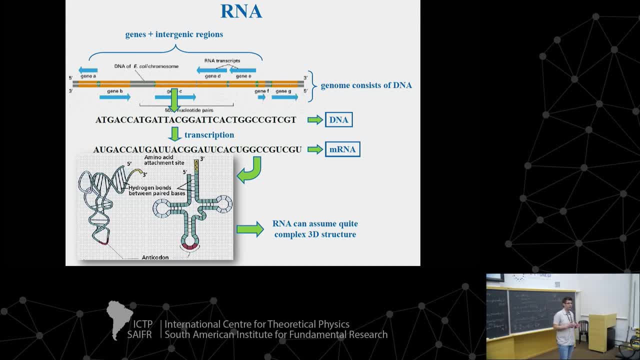 is interacting with, for example, some protein. it is this shape of RNA, that is its secondary structure, which is crucial. And actually, for those of you who are bioengineers, you might have heard the term optomer, So optomer is a short piece of RNA. 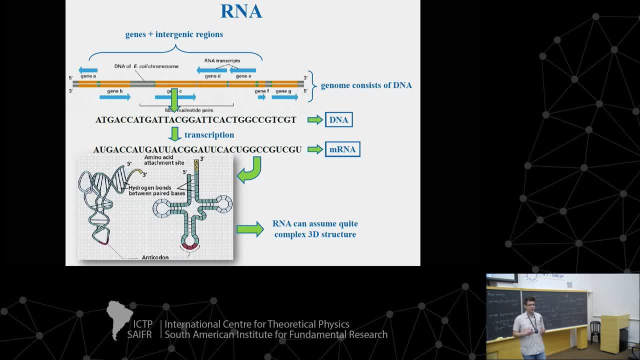 And in Greek optos means shape. So what is meant by that is that interactions of RNA with other things in the cell are really determined by its shape, by its secondary structure. So even as an approximation to view RNA as a one-dimensional sequence of latter. 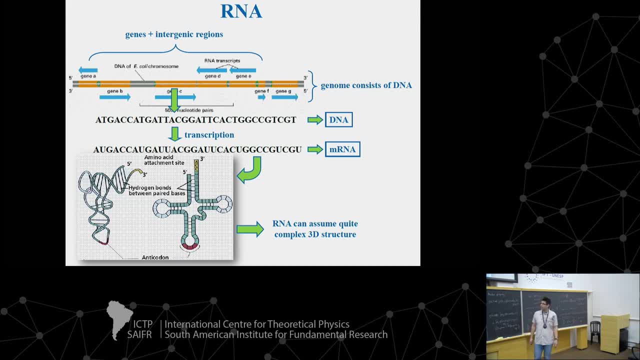 it is not even a good first approximation. And then of course RNA can have the tertiary structure. For example you can have quadruplex RNA and things like that. But you know, mostly it is the secondary structure which is most important as far as RNA goes. 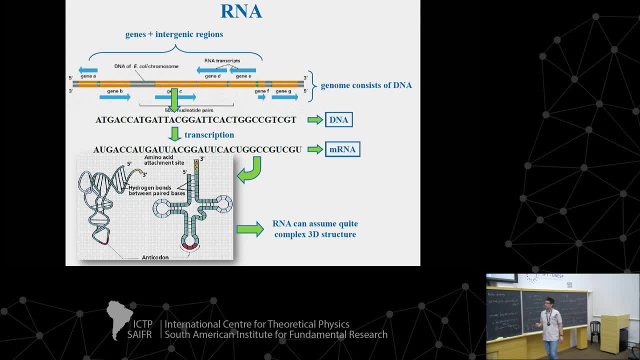 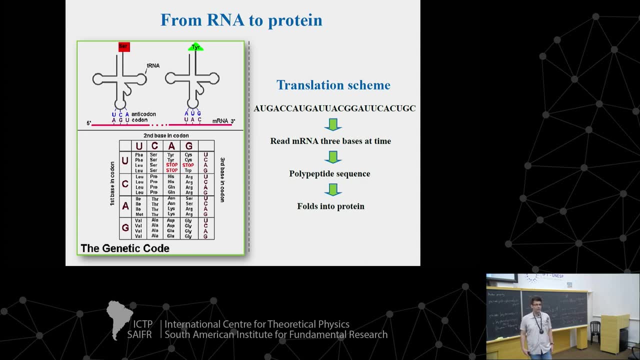 And there are a number of methods in bioinformatics which predict secondary structure of RNA. Now, finally, we come to translation in this central dogma. So I do not have much to say about translation. So we start from the start, codon. 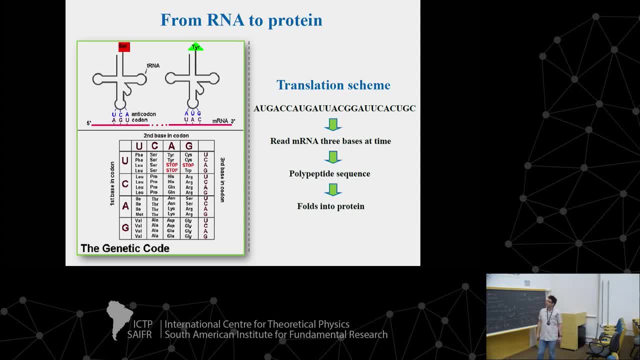 You end with stop codon And then you read DNA as triplets, which means that three bases at messenger RNA. they determine the amino acid to which it will be translated, And then you get polypeptide sequence. This polypeptide sequence then gets folded into protein. 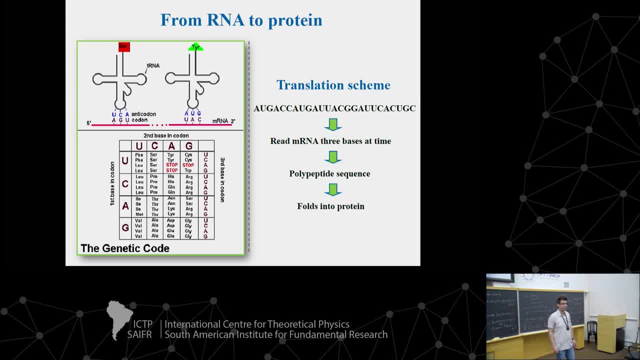 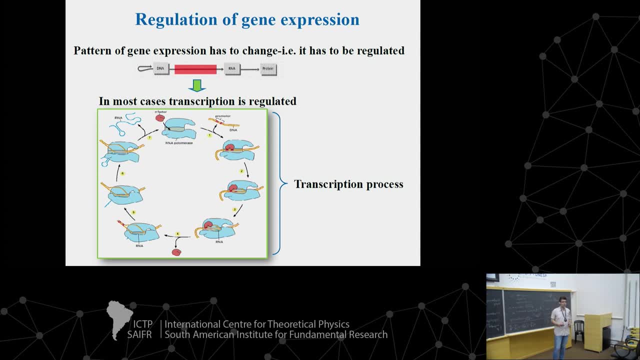 And again, you have heard much about this already, so I will not go into that. OK. But now, as I mentioned, what is really important for systems biology is regulation, And not only for systems biology, but for biology in general. 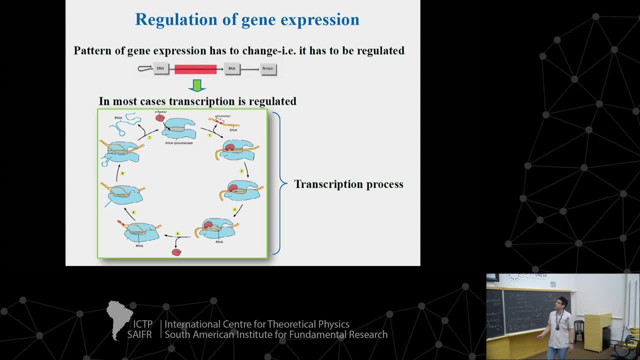 And so the most important point of regulation is transcription. And here is given a sequence of simple scheme of transcription. It applies to bacteria, but then conceptually it is sort of similar thing in eukaryotes as well. So what happens is that you have one large molecular motor. 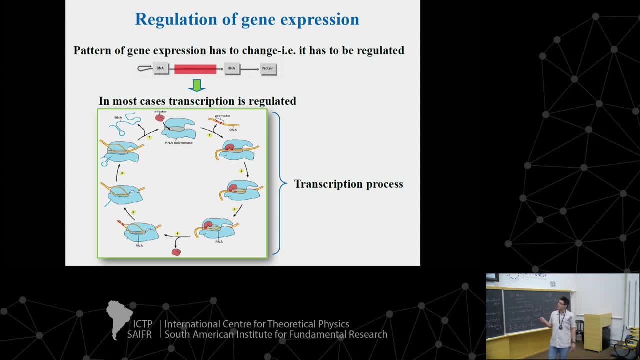 It is called RNA polymerase, And then what happens is that RNA polymerase binds to DNA. When RNA polymerase is bound to DNA, then the two DNA strands get separated, And that is why I mentioned that even at basic level, the structure of DNA can be important. 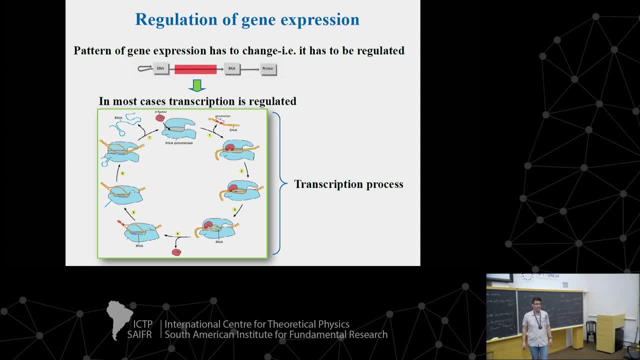 For example, here we have melting of DNA. The transcription will not start unless the two DNA strands are separated. Then once you separate the two DNA strands, then transcription can initiate, meaning that RNA polymerase leaves the promoter RNA starts to be synthesized. 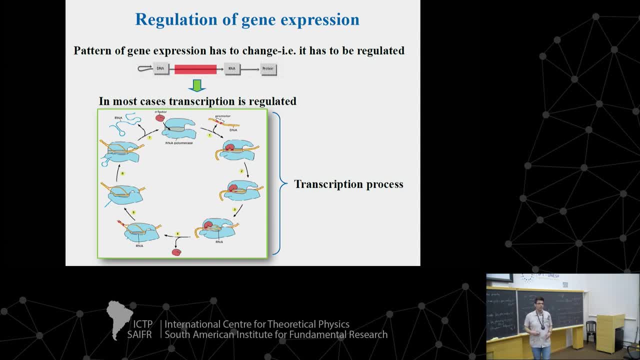 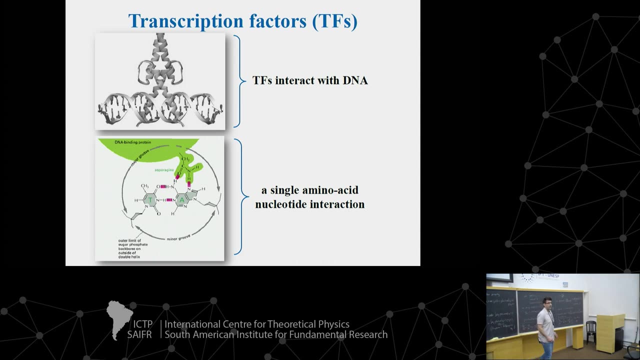 And then you have RNA, And then we are back to the center of dogma. From RNA you get protein and so on. So this is the basic process, But then this basic process is very often regulated, And it is regulated most often by proteins. 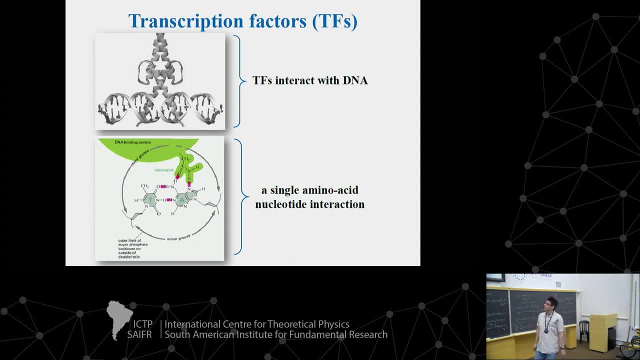 These proteins are called transcription factors, And what these transcription factors do is that they interact with the DNA. So interaction is by amino acids, which are being which interact with DNA, with bases in DNA, And here is shown one single amino acid. 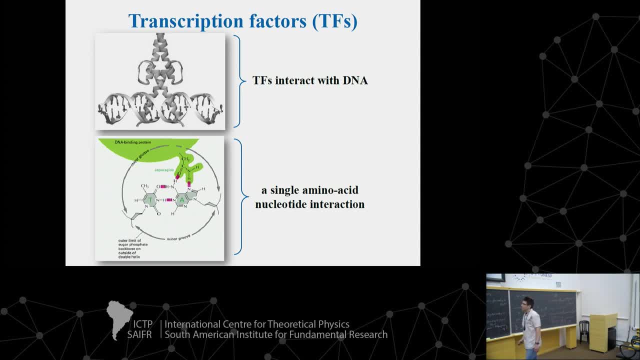 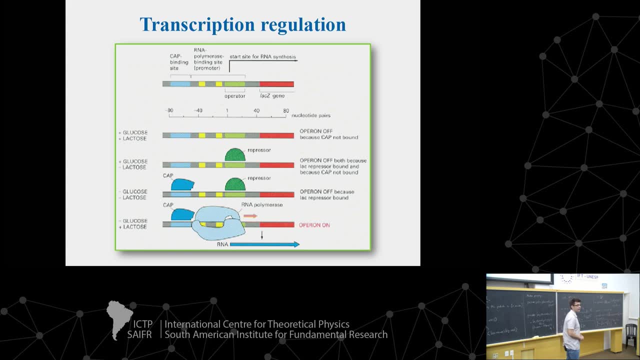 which is making interaction with one nucleotide. So this is sort of on a small scale And then on a larger scale. this is one classical example of how regulation of transcription works. It is so-called Lac operon, And basically molecular biology sort of started with Lac operon. 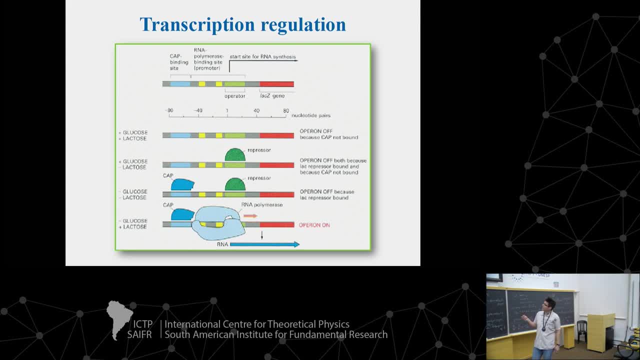 So what is shown in red here is a gene, And this gene codes for enzyme which degrades sugar, which is called lactose. Now, as bacteria goes around, it must eat, So it is searching for food, The preferable food for bacteria. 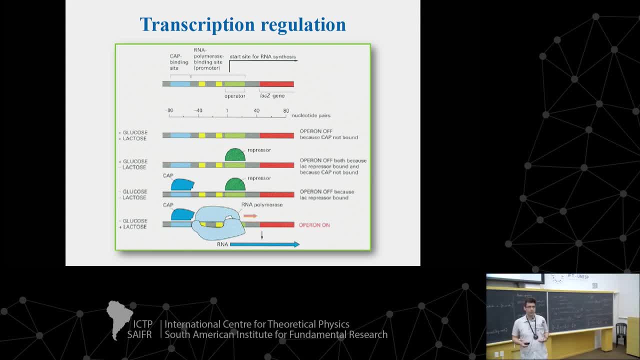 is sugar called glucose. So whenever there is glucose around, the bacteria will eat glucose. But then if there is no glucose, bacteria gets hungry and it has to use other sugars. So one alternative sugar that bacteria can eat is lactose, And this enzyme actually degrades lactose. 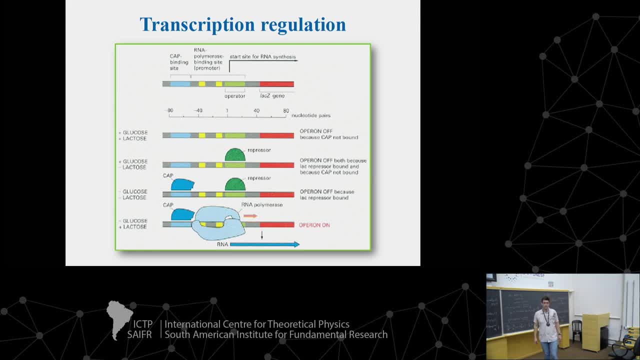 and it allows bacteria to eat when lactose is present. But now this process is regulated, So, for example, when lactose is absent, what happens is that there is a transcription factor, which in this case is receptor, So it is shown by this green thing here. 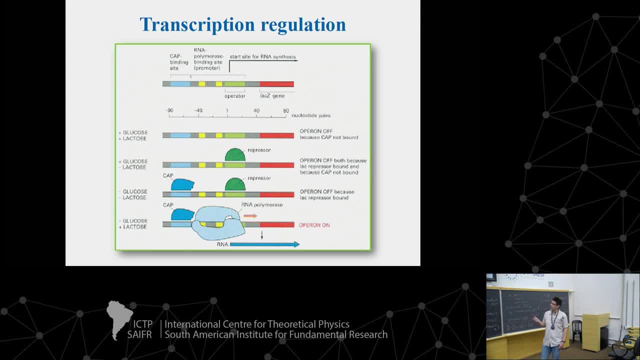 And then this receptor is active, It will be bound to DNA. Now, when receptor is bound to DNA, RNA polymerase cannot bind to DNA and the gene will be off Meaning. if you do not have lactose, there is no need to synthesize the enzyme. 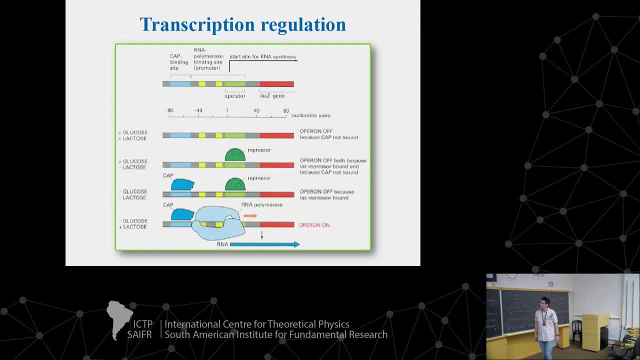 it will be in lactose, So you know the gene will be off. There is another transcription factor here. It is shown in blue here And it is acting as an activator of transcription. So when the glucose is absent, meaning when the bacteria is hungry. 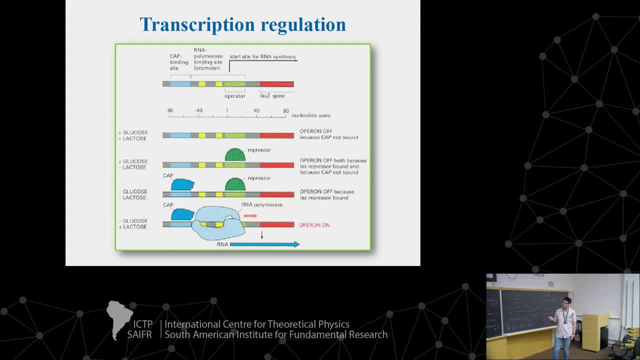 this transcription factor, this activator, will be bound And what it is doing is that it is recruiting RNA polymerase to the promoter. So then you have RNA polymerase bound to the promoter And when you have the transcription, the gene is being synthesized. 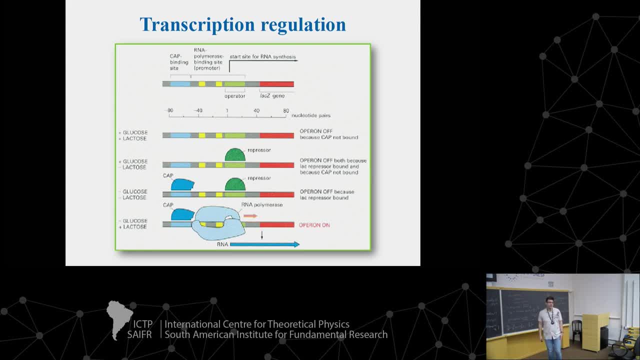 The gene is off, The gene is on there. So, in summary, you will have the transcription only if the glucose is absent, meaning if bacteria is hungry. And if lactose is present, that is, if it should be degraded, then RNA polymerase will be bound to the promoter. 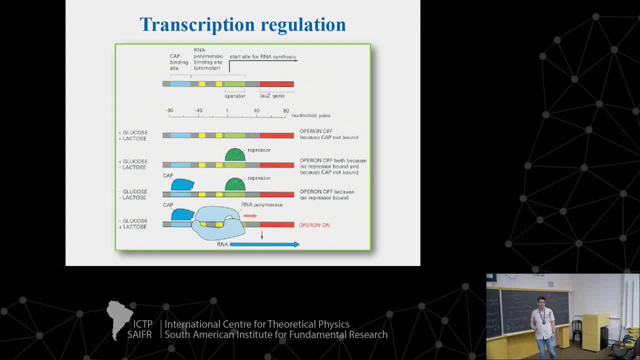 Transcription will start and then appropriate gene- in this case protein which is degrading lactose- will be synthesized. So this is a nice example about control at the level of transcription, And what I should mention is that this is on the level of single genes. 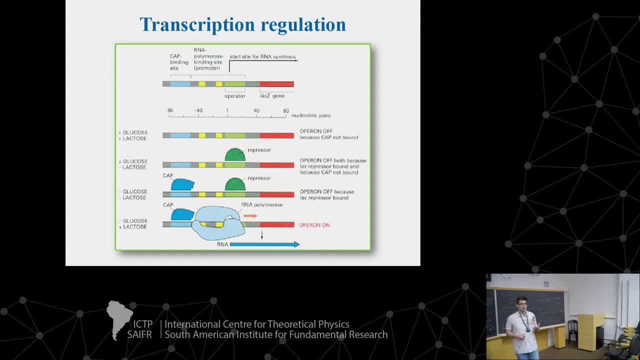 But now imagine this one transcription factor: this one gene can regulate another gene, and then this another gene can regulate some other gene, and so on. And by doing this you really have a network. You have a network of genes which are connected with each other. 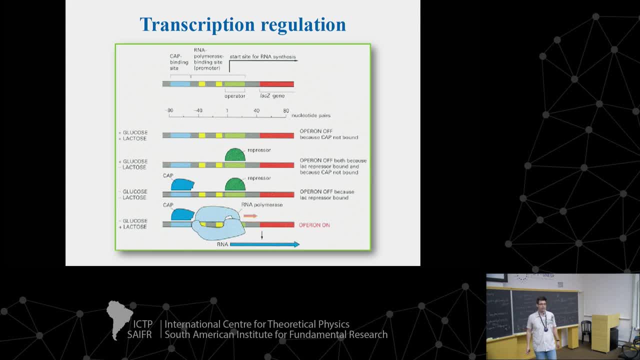 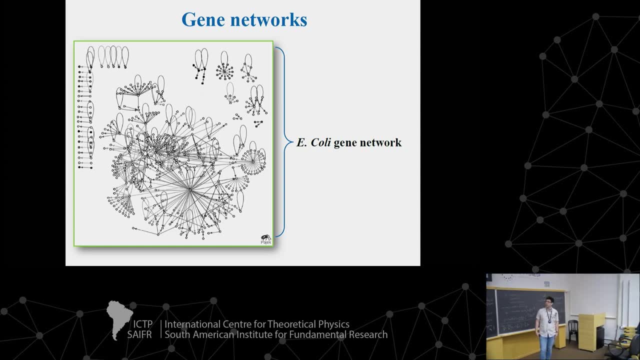 And being connected means, in this case, being regulated by each other, And then by having this, you have what is called what people call gene networks or gene regulatory networks. For example, this is here is shown: gene regulatory network for bacteria. 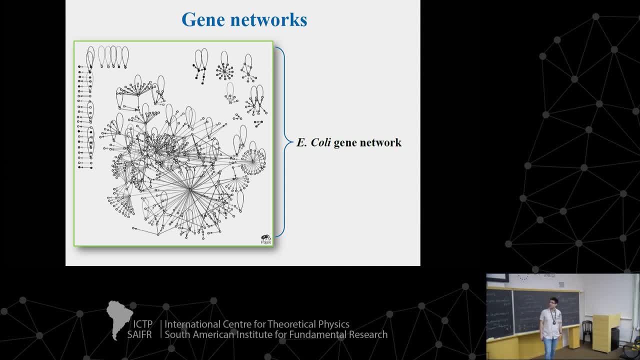 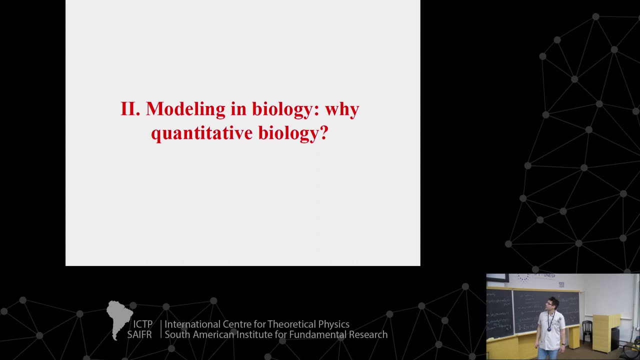 which is standard bacterial model system. So just briefly, these circles here are genes, and then these arrows means regulation. So if one gene is regulated by another, you have an arrow, If not, you do not have. Okay, So this was sort of 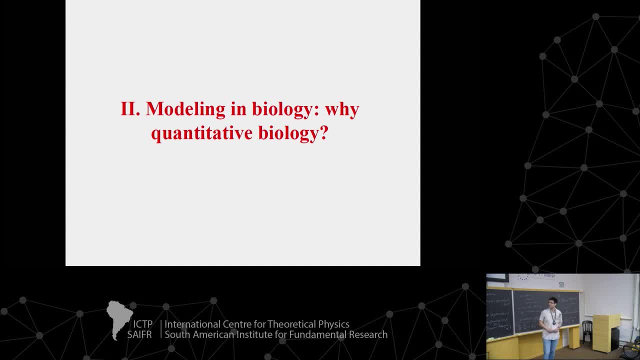 introduction in what we need, as far as this lecture goes, in molecular biology. And now, since this is introduction lecture, so one question is why we need quantitative biology, Or why we need mathematical biology, Or why we need mathematical modeling in biology. So actually, 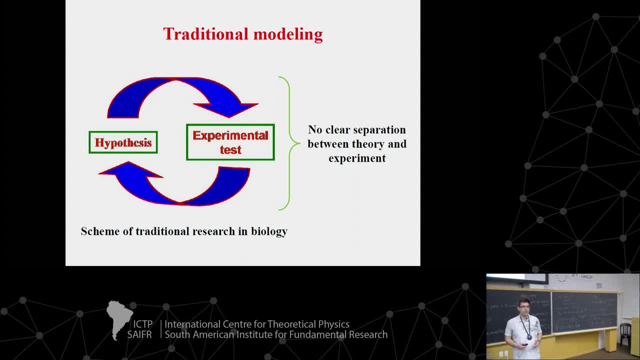 when we talk about models, what I should mention is that modeling is very much traditionally present in biology. It was always present, It was always there, And this is sort of traditional cycle of knowledge, so to say. in biology You start with some hypothesis. 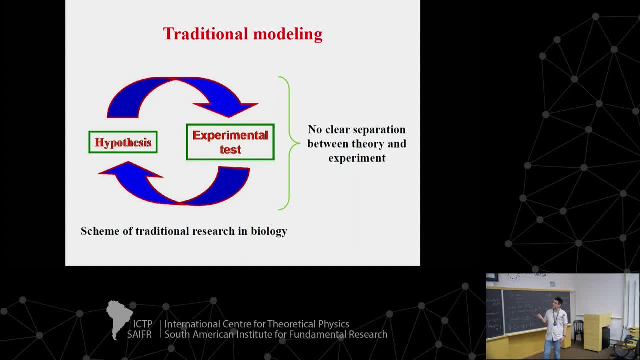 And then, starting with hypothesis, you do some experimental test. By doing experimental test you can well. the answer can be either positive or negative. So then you refine your hypothesis depending on the experimental test, And then it goes on and on. 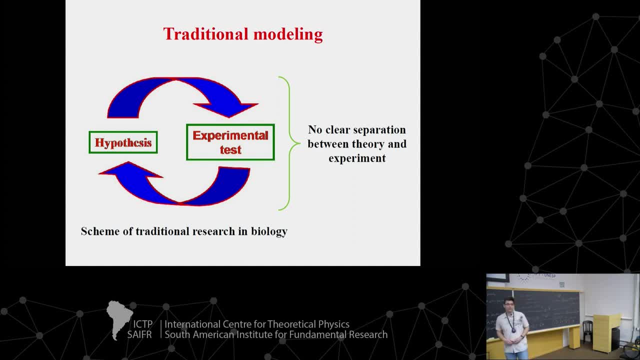 Now what you should mention here. so the model is present here, but first of all, model is qualitative rather than quantitative, And then, secondly, there is no clear separation of work between theory and experiment, which would be characteristic for physics. 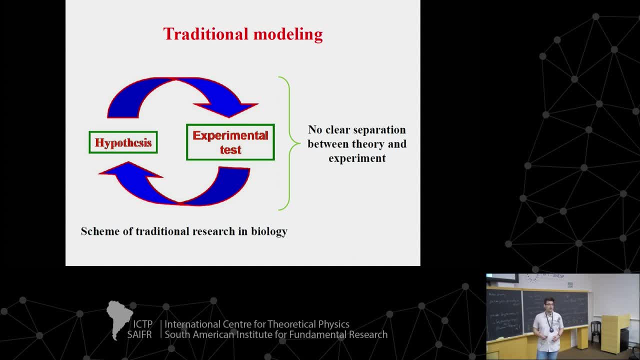 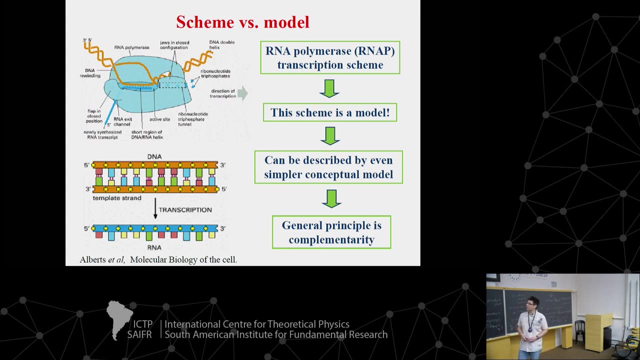 In other words, experimentalist, is his own theorist at the same time. So he's the person who is both formulating the hypothesis and doing the experimental test. And actually, if you open any molecular biology book, you will find a number of nice models there. 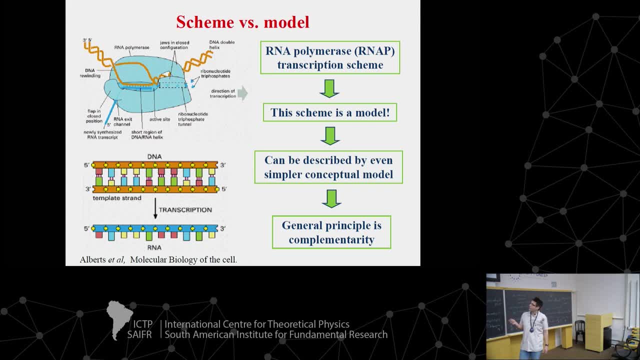 For example, I was mentioning the description, and this is figure taken from one classical molecular biology text and it very nicely summarizes understanding of transcription. So what happens is that you have RNA polymerase. it is a large machinery. it moves along the DNA. 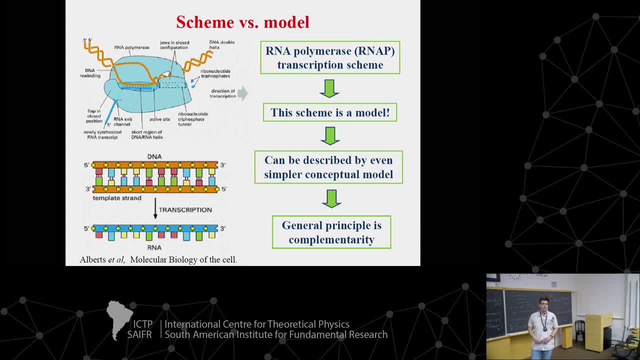 it separates the two DNA strands and RNA is being synthesized. So this is model, And even more you can make this model even more simple. So you can say that transcription works by having one of the two DNA strands serving as a template and then by serving as a template. 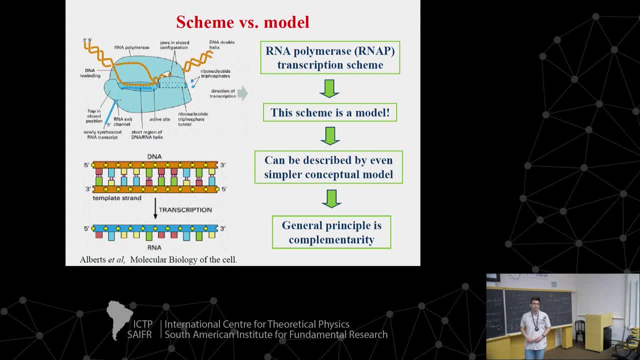 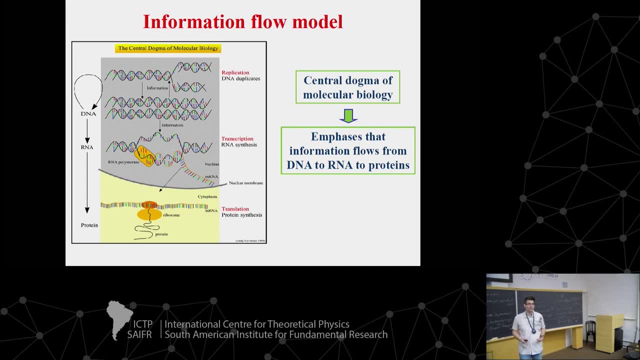 you synthesize RNA to be complementary to one of these two DNA strands, And also the central dogma I was. I mean you heard about central dogma several times up to now. It is also a model. It is a model of how information flows. 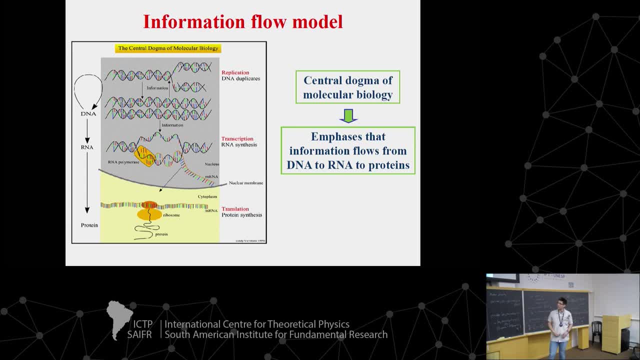 It tells you that information flows from DNA to RNA, to protein, Although, as I will mention briefly, this model is actually very much insufficient for systems biology. What is not present in this model is regulation or feedback loops, And feedback loops are really very important. 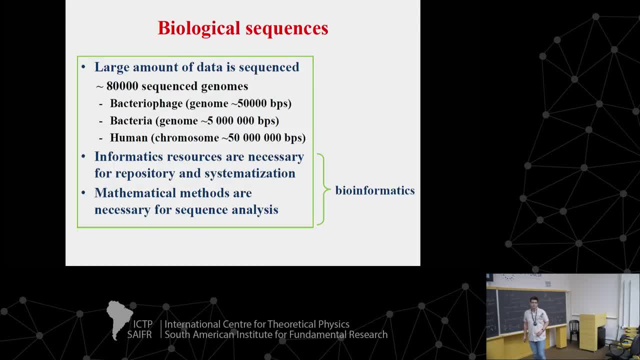 So soon I will come to that. OK, now then, what has changed? So I mentioned that very much. always you had models in biology, But then there is something what people call the evolution in molecular biology, And this revolution is that now, at some point, 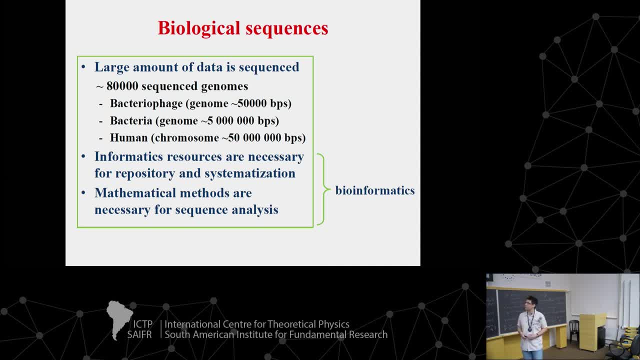 a really large amount of data started to be accumulated. So if you look at gene bank, for example, today you have about 80,000 completely sequenced genomes. And if you look at lengths of these genomes, for example, if you look only at virus, it is about 50,000 base space long. 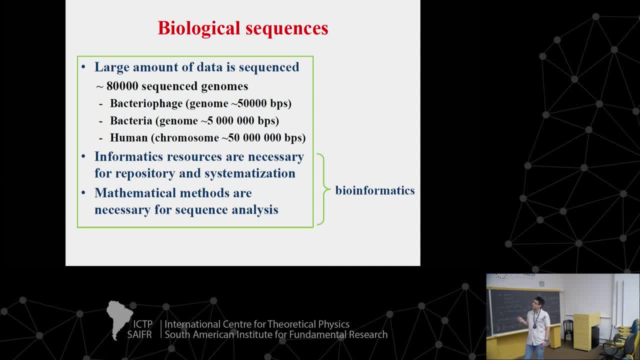 If you look at the bacteria, it is two orders of magnitude longer, So typical bacteria genome is about five million base pairs. If you look at a single chromosome in human, it is order of magnitude longer than bacterial genome And there are 23 chromosomes. So you see that the total length is about again two orders of magnitude larger than bacteria. So just to get some sense, if you would like to write the bacterial genome in a book, you would need a book which would be 1000 pages long. 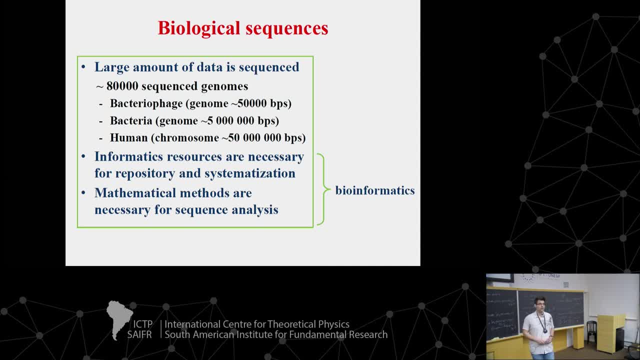 And then if you would like to write human genome, then you would need 1000 of such 1000 pages long books. So then it became obvious that you need resources in order to have repository of this information and to somehow make systematic this information. 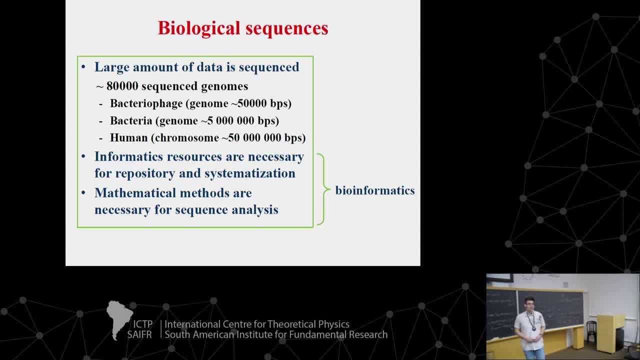 And this is what are now biological databases, And also, in addition to databases, to just storing information. you need some way in order to make sense of this information, And for this you really need mathematical methods. So you cannot just take, I don't know, five million base pairs. 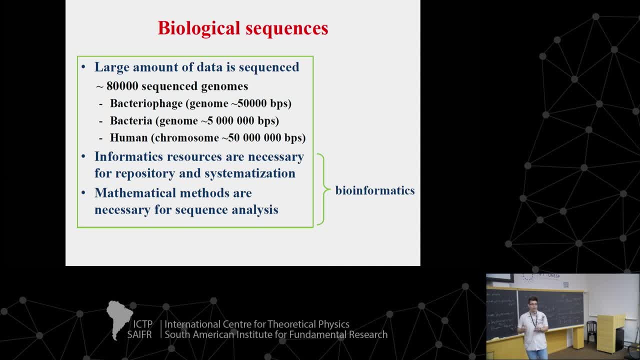 You cannot write them, stare at them and say you know, here are functional parts, here are not functional. You need some way to process this information And, in one word, basically these methods for storing this large amount of information and for analyzing this large amount of information. 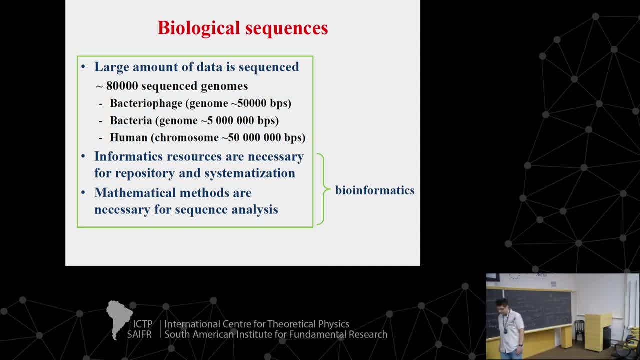 it's. it's called bioinformatics. So nowadays bioinformatics is mostly done, I mean logically- by computer scientists, by statisticians very much. But actually biophysics has a very important role in bioinformatics as well. And actually, if you look historically, 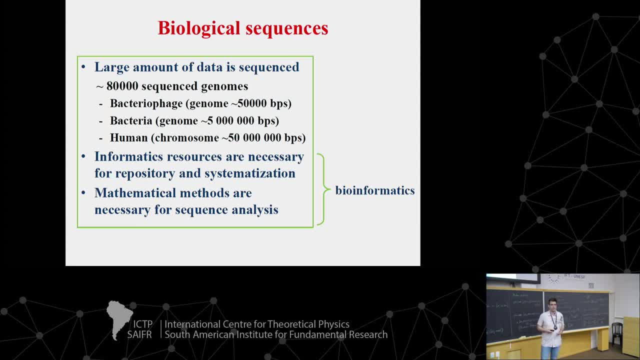 bioinformatics in fact started from sort of biophysics. Even now, if you look at the National Academy of Sciences, the appropriate section is called biophysics and computational biology. So the reason is because computational biology basically started from biophysics, which makes sense because in the beginning, 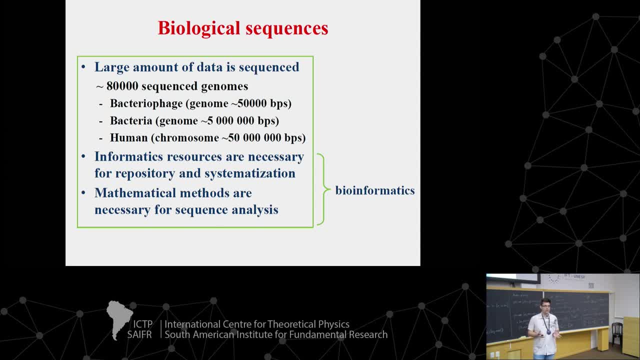 people were thinking: you know how physically, say, RNA folds, how protein folds. They were thinking about interactions between proteins and DNA in order to understand regulation and so on. Now, with complexity of data, it also very much moves towards computer science and towards statistics and so on. 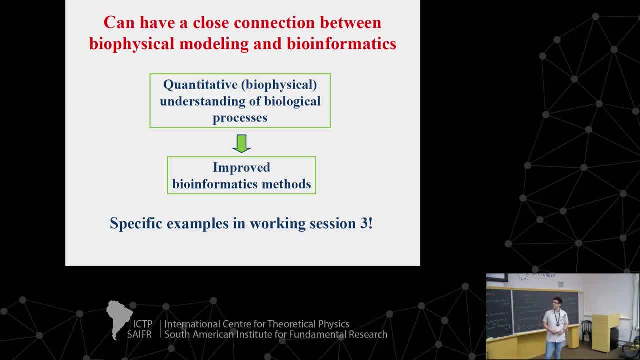 But, as I mentioned, so bioinformatics can. biophysics has very important applications in bioinformatics as well. So the basic idea is: if you have, if you can understand biophysically how some processes in the cell is happening, then you can improve or make a new method. 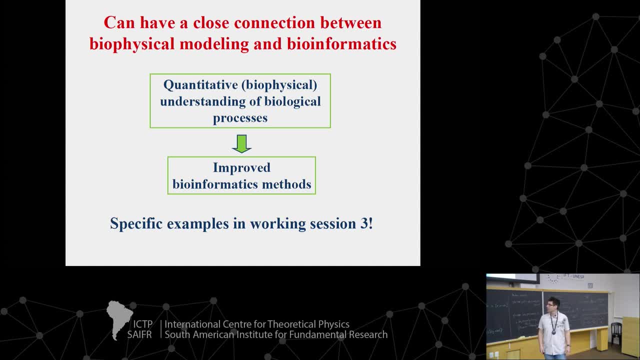 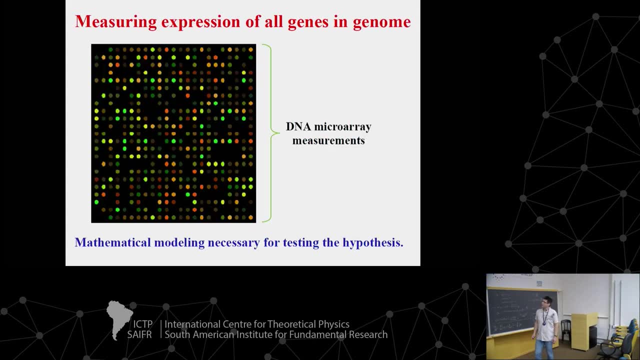 which is analyzing the appropriate data, And I'll talk more about specific examples in this third working session. OK now, in addition to just having this large amount of sequence data, another thing also became possible, And this thing was to quantitatively measure essential expression of genes. 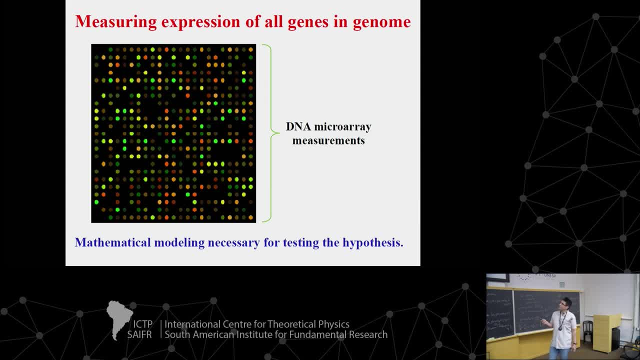 So what is shown here is the DNA microarray. So basically each spot on DNA microarray, say, corresponds to one gene And then intensity of these dots here they tell you about to what level this gene is expressed in the cell And this means that to every gene that is. 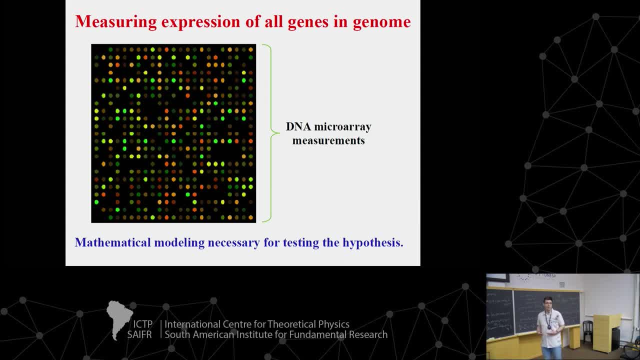 to every dot you have one number associated and you have really many genes. For example, even in bacteria, you have something like 5000 genes in alkyl. it's much more than that, and so on. So this means that on one hand you have numbers and then on the other hand you must test your hypothesis. 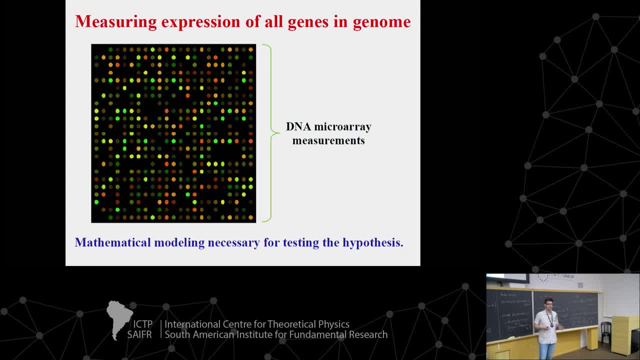 So you can really not compare numbers with words. You cannot compare numbers with qualitative models or qualitative hypothesis. You must have quantitative models in order to compare numbers with numbers, so that you can test hypothesis, And this is one reason why mathematical modeling became really necessary. 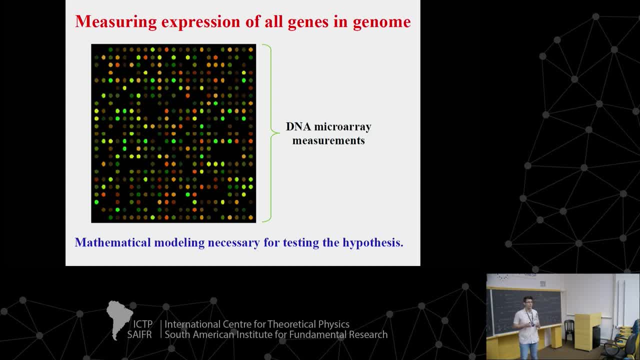 And I should also mention not only that you can measure expression of genes, but you can do it under different conditions, you can do it at different time points. you can now do it at the level of single cells, at the level of the entire population, and so on. 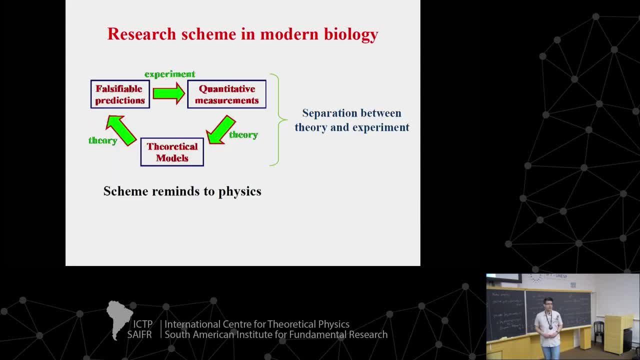 OK, so now with this we come to sort of more elaborate research cycle which is associated to sort of this revolution in molecular biology. So you start from, you know theoretical model, and then this model is hopefully making falsifiable predictions. Then these predictions are being compared with experiment. 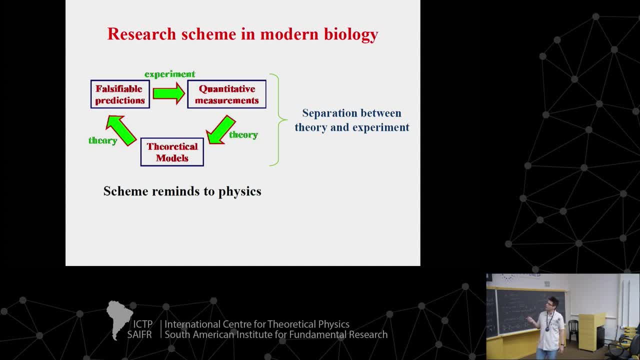 And, as I mentioned, you basically need to compare numbers by numbers. So the experiments are now quantitative measurements. Then, depending on the outcome of this comparison, you will modify the model Again, compare things and so on And now. So this shim very much reminds to the shim in modern biology, very much reminds to physics. 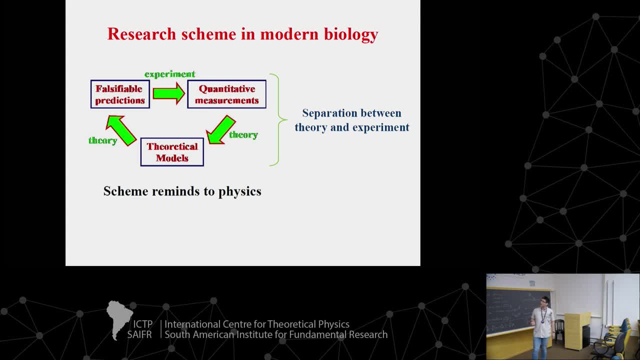 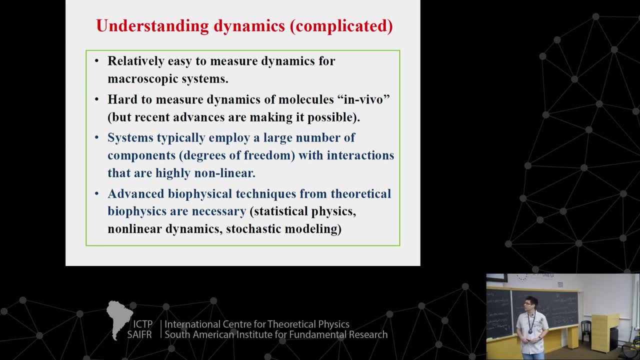 And I should mention actually one more thing, And this is related with, with basically the second lecture that I will go through tomorrow. So, in addition to having just quantitative measurements, what also happens is that measuring dynamics at the level of cell It's not easy, It's not trivial. 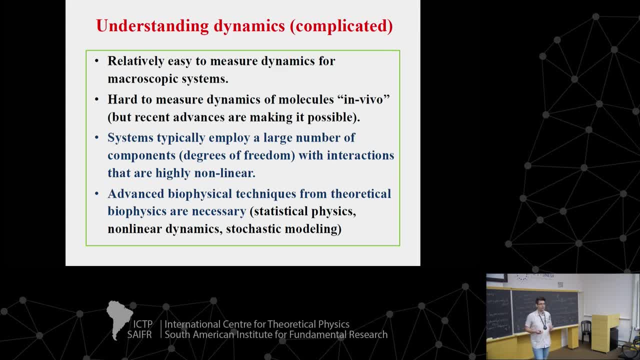 It's much more hard to do than measuring dynamics in in in macroscopic world. So, for example, if you need to to measure, if policemen has to measure speed of the car, he can now this do this easily. But then measuring dynamics of molecules inside cell. 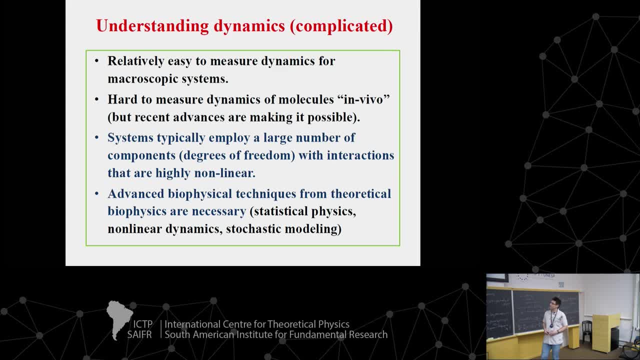 It's. it's. it's not true, It's not trivial at all, although it's. it's possible by mainly Today, by by advances in spectroscopic techniques. But then, in addition to that, the system which you are dealing is is really complex, and it's complex in two ways. 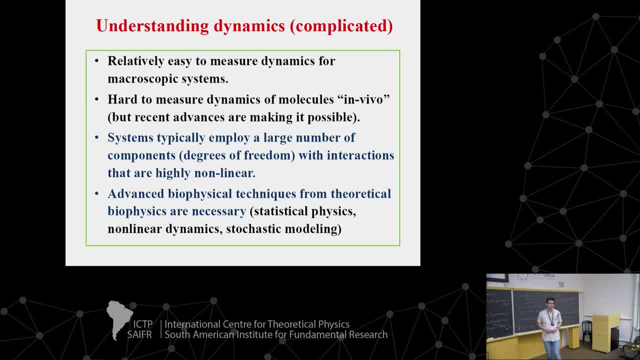 It employs a large number of components, large number of degrees of freedom. So I was talking about transcription factors and as and the regulations of one transcription factor is present in many copies, It can be from few transcription copies of transcription factor in the cells to few thousands. 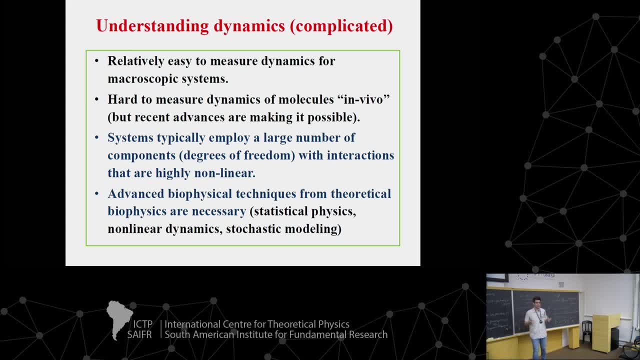 And, moreover, you do not. You have only single transcription factor, You have many of them in the cell. So which means system has many degrees of freedom, and natural way to treat this Many degrees of freedom is to use statistical mechanics of statistical thermodynamics. 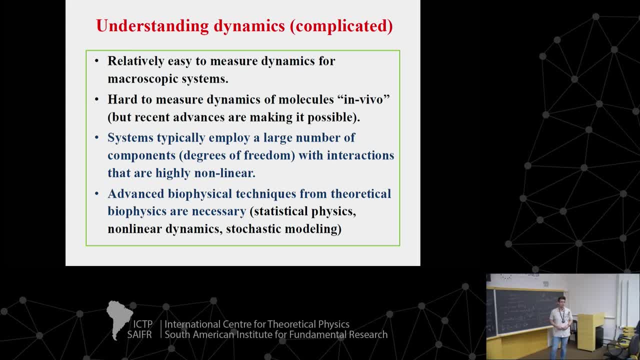 And then, secondly, interactions are also highly nonlinear, And this will be basically what the rest of my lecture today will be: Why this nonlinearity is really inherent when you're looking, looking At this- to the systems at the molecular scale. So 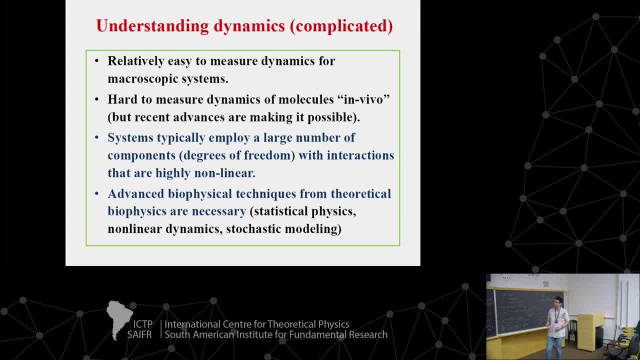 in addition to having quantitative measurements, then you also need a sort of advanced biophysical techniques in order to develop appropriate model. So they include statistical physics, nonlinear dynamics, stochastic modeling. I will not actually call it stochastic modeling in the sense of of of of systems biology during these lectures. 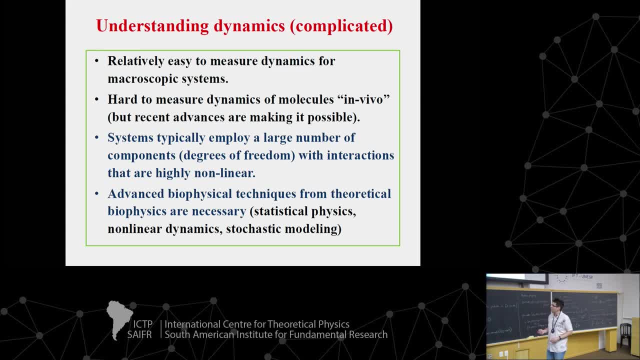 But OK, and I should mention one more thing. So I was. I was mentioning different techniques that you used, but actually very often the hardest thing when you are making quantitative model is actually biology. So when you come to equations, this can be the easier part. 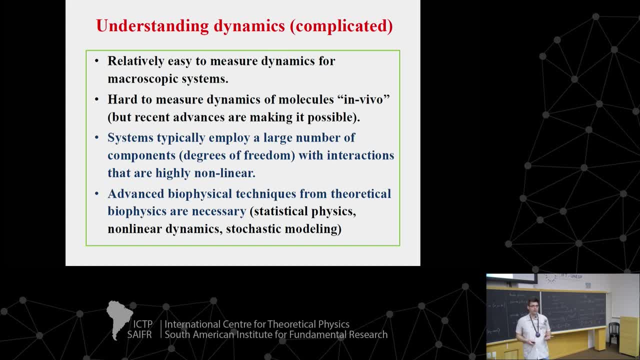 But very often the most hard part is to first understand your system, to understand the experiment behind it, to get the appropriate numbers. And so many people who, who, physicists, who are doing biology, they say that if you want to do biologists, you, you should really become biologists. 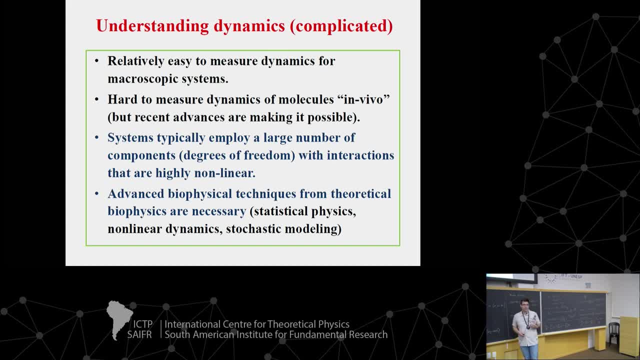 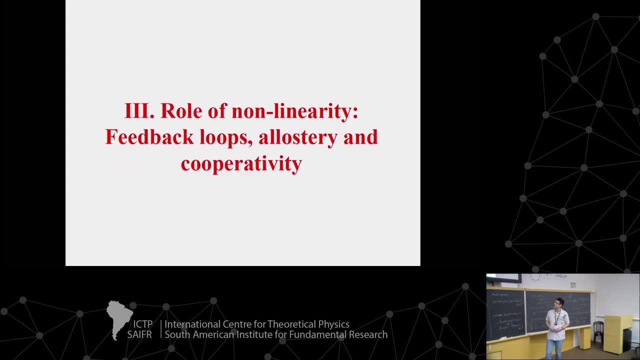 And it also applies the other way around. So, for example, we have seen Chuck Farah here who is biologist, biochemist, And and well, obviously he had to also come into physics. very much OK, and with this I will, I will, I will conclude this sort of general part. 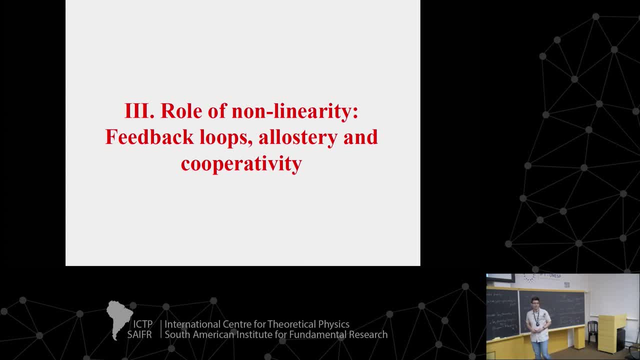 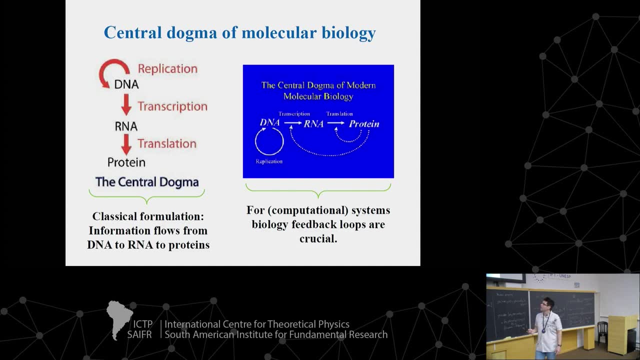 And now the remaining thing. It will be why, why non-linearity is so important when you look, look at at systems inside cell. So again, this is the third time that I'm showing the central dogma, But what I mentioned is that the central dogma is insufficient for systems biology. 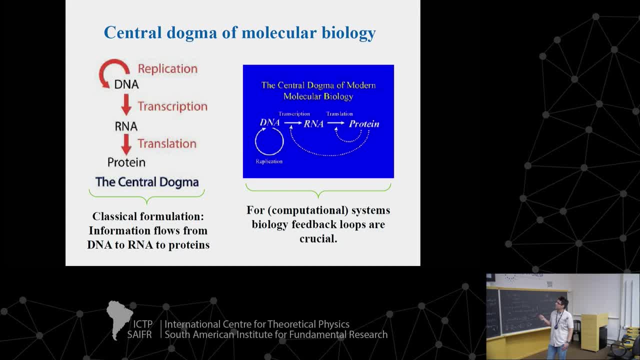 What is really essential are these feedback loops. So I already gave you one example of the feedback loop. So this is regulation at the level of transcription. So proteins come, for example, to transcription factor and then they regulate this process of synthesizing RNA from DNA template. 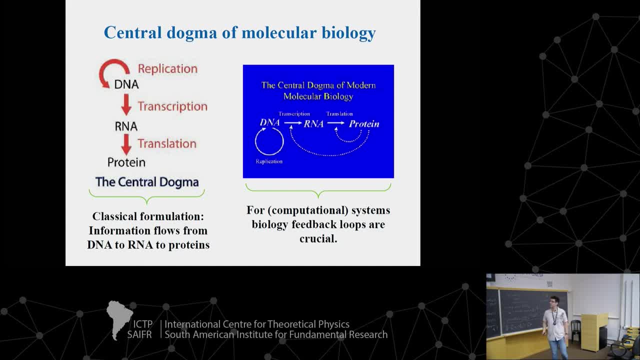 And this is not the only feedback loop that you you can have. For example, you can have proteins regulating translation as well, for example, degrading RNA. Actually, I will give you one example about this. I think tomorrow you can, you can have RNA also regulating transcription. 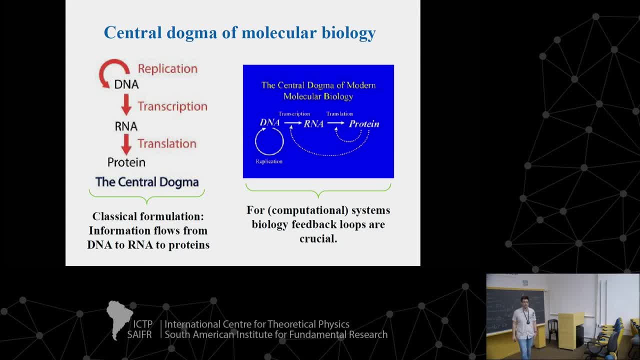 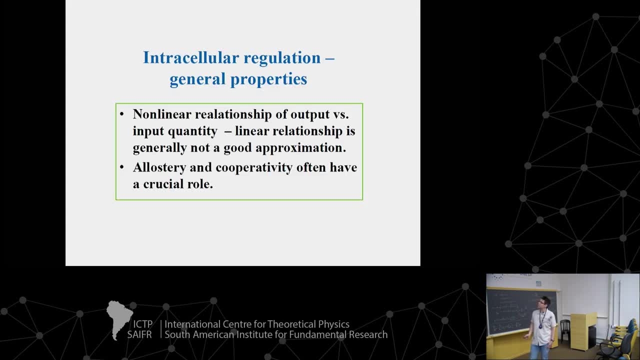 These are so-called small RNA or micro RNA molecules, which are also a very hot topic, and so on, But this, this feedback loops, they're really essential for for systems biology. So the point that I want to make is that, even as the first approximation, 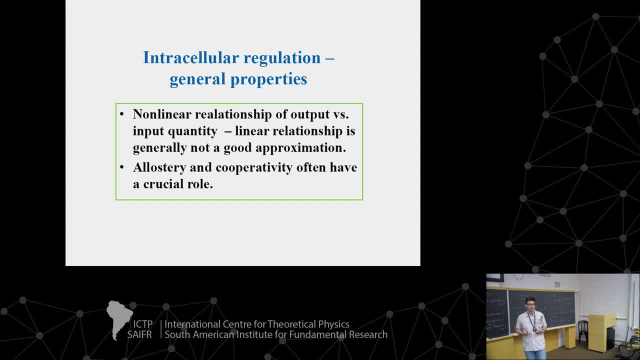 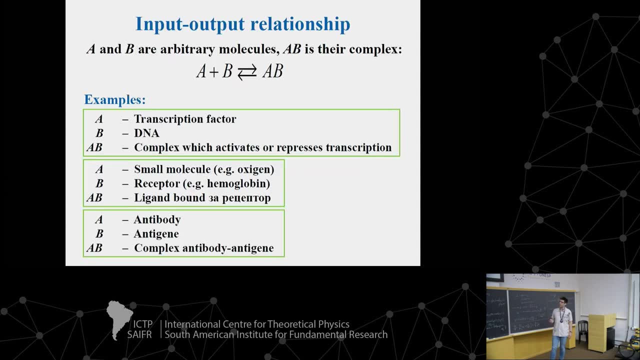 treating your system linearly at the, at the intercellular level is is in most, most of the cases, insufficient. And basically, why is that So? even if you look at the most elementary process, so we have molecule A which is being bound by molecule B. 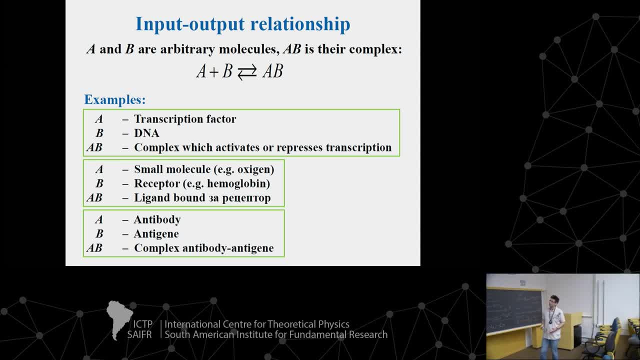 So then we have this complex AB, And there are many examples. For example, A can be transcription factor. in this example that I showed you, B can be DNA. Then AB is complex between transcription factor and DNA. Or AB can be, for example, A can be some small molecule, for example oxygen. 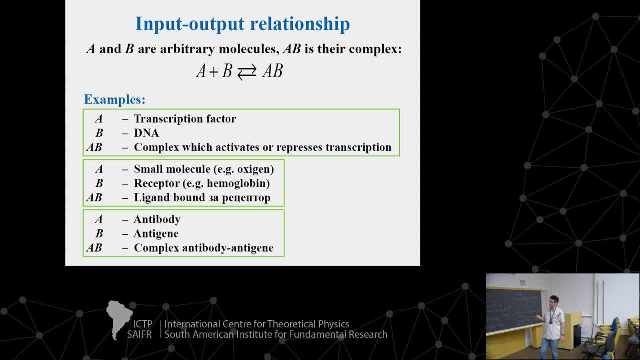 B can be some receptor, for example hemoglobin, And then AB can be ligand bound to this receptor or, in A and B, for example, can be antibody and antigen and they can make a complex. But this is sort of a very fundamental. 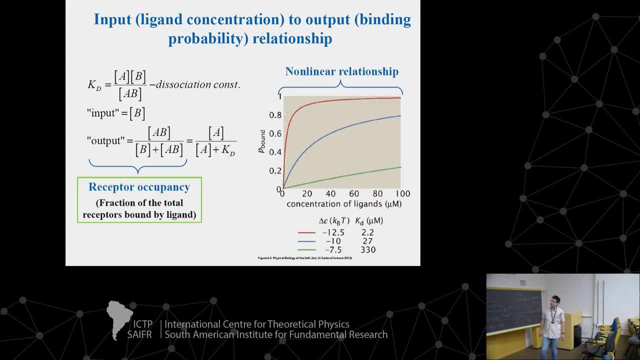 process at the level of interaction of molecules inside the cell. So when you have equilibrium, this is the dissociation constant for this process. So you get dissociation constant, but you're just multiplying concentrations on the left hand side and dividing this by the concentration on the right hand side of the reaction. 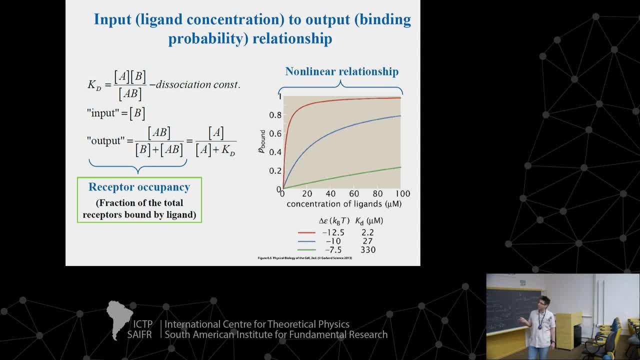 And then let me say that our input- I'm sorry, here's a mistake, It should be A- So our ligand is concentration of our ligand is input, And then output is how much of the receptor is being bound by the ligand. 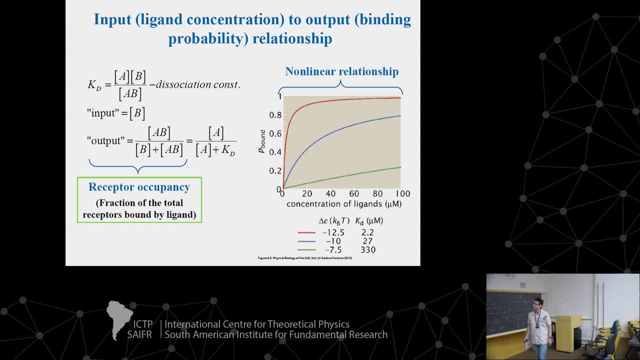 So it is fractional occupancy of the receptor by the ligand. So here is the number of receptors which are being bound by the ligand And here is the total number of receptors. So this is our output, again fractional occupancy of the receptor. 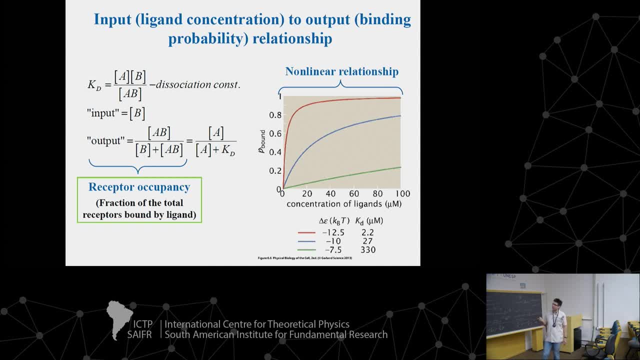 And then if you use this relationship for the dissociation constant, we get this input to output relationship. So again, A is our input, This is our output. And then if we plot this output versus input, fractional occupancy as a function of the ligand concentration. 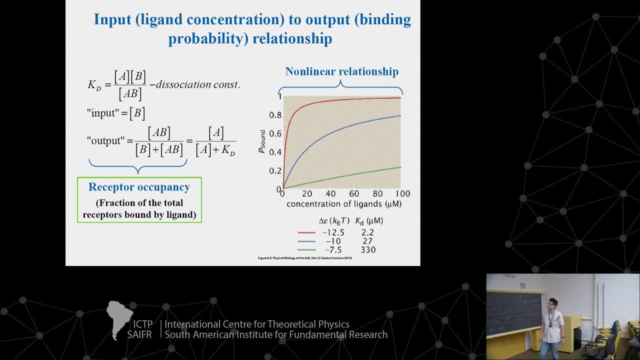 What is what we see is that even here, at the most elementary level, this is a nonlinear curve, this is sigmoidal curve. And actually, this dissociation constant, it defines the concentration of ligands at which the receptor is half saturated, meaning it's saturated 50 percent of the time. 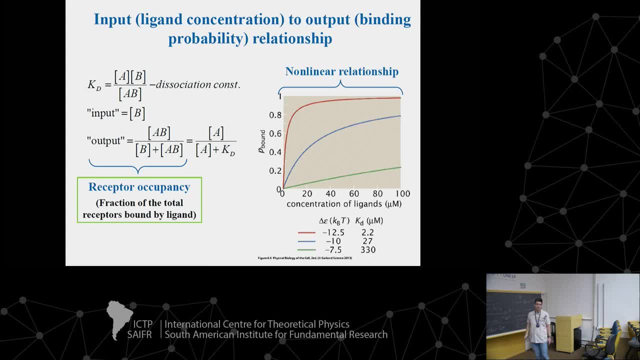 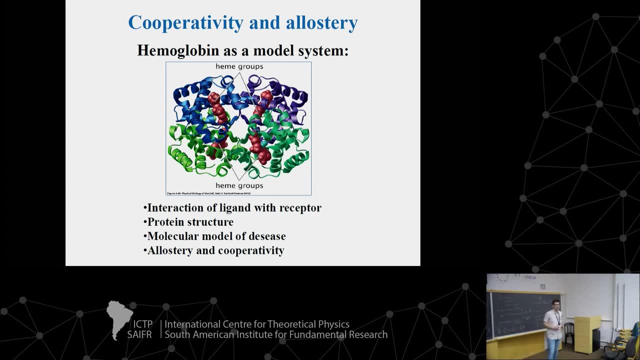 So, for example, look at this red curve. It's evidently nonlinear. And actually not only that. very often, cooperativity is important and comes in in biological systems, And one classical example is hemoglobin. Actually, hemoglobin is a model system for a number of things. 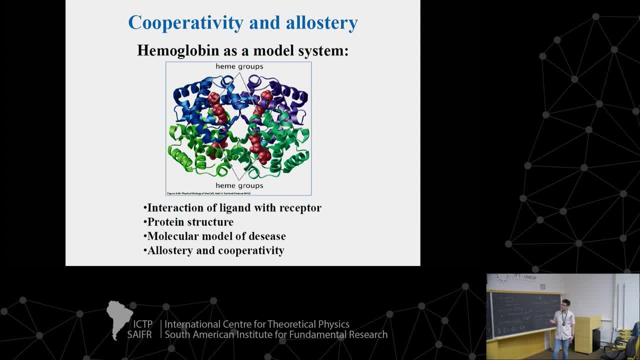 You already heard that it is a very nice model system and historically has been a very nice model system for protein structure. Then it is a model system for interaction of ligand with receptor, where ligand is oxygen and receptor is hemoglobin itself. This is the example that I will give. 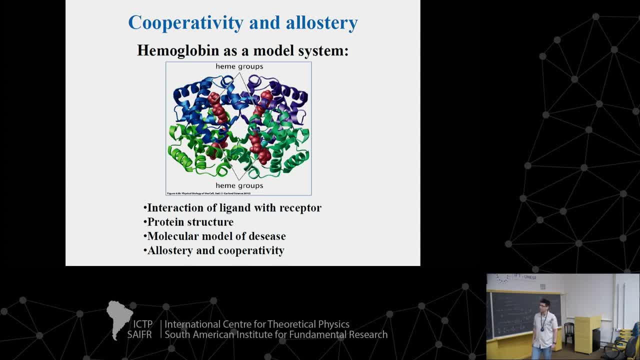 It is also a model for molecular model of disease. It is sickle cell anemia and it is actually disease when you have mutation in the hemoglobin gene and which makes the protein dysfunctional. And also importantly, it is a model for cooperativity and allostery. 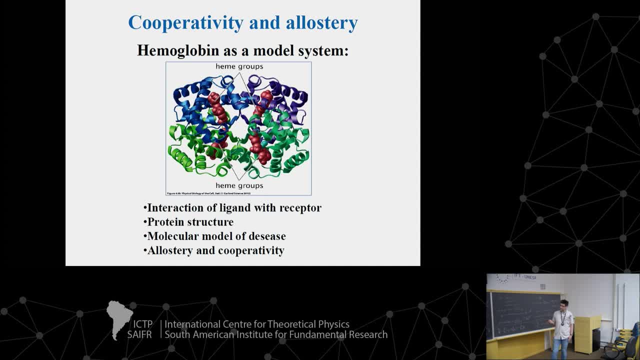 So now, what is meant by allostery? So here, on hemoglobin, you have four binding sites for oxygen And what happens is, if only one oxygen molecule will be bound to hemoglobin, you will have a conformation change in the protein. 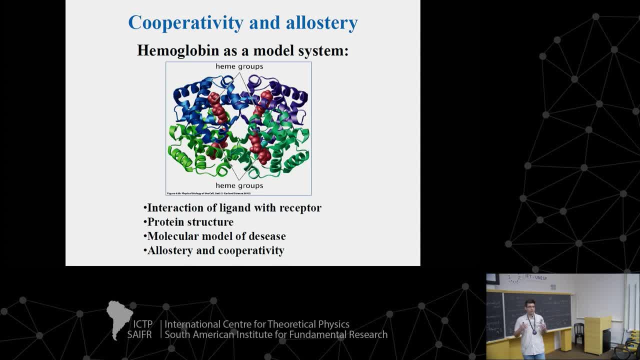 And this conformation change will lead to the other three oxygen molecules being able to bind much more easily. So essentially, as soon as one molecule will bind, the other three molecules of oxygen will also bind to hemoglobin, But notice this. So this is an example of cooperativity. 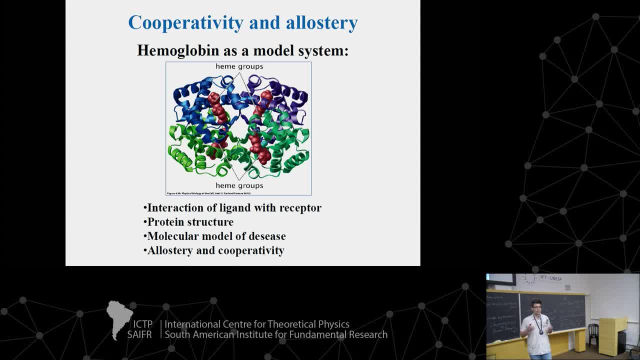 But notice in this example, this cooperativity does not happen through direct physical interactions. So these oxygen molecules, they do not physically interact with each other, But as soon as one binds, it will include the other three molecules. And there are also evidently other ways to achieve cooperativity. 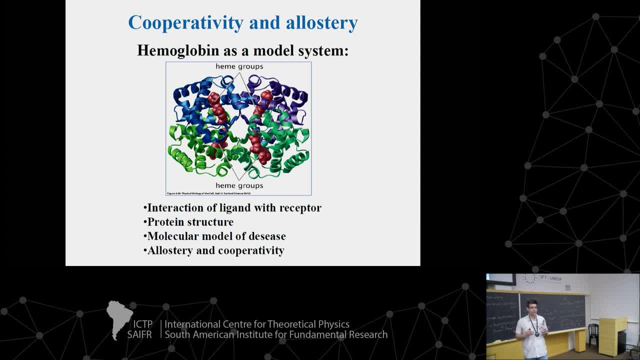 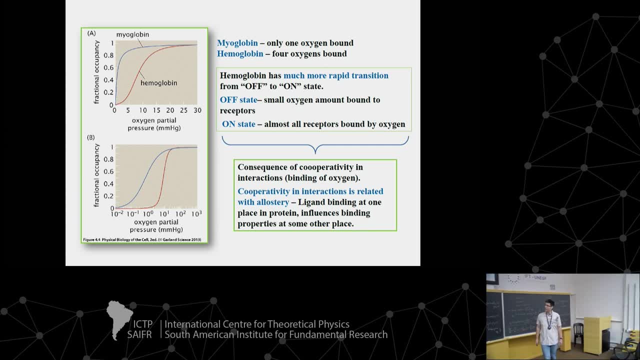 You can have also direct physical interactions between molecules, And I'll give an example. You can help us later about that as well. But now let me look at the binding curves. So what is shown on the vertical axis here is fractional occupancy of hemoglobin, in this case. 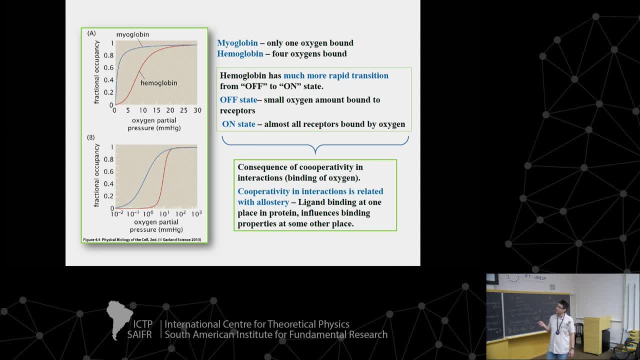 And here on the horizontal axis is given concentrations of ligand, meaning oxygen. Actually, here the pressure of oxygen is given, which is obviously directly related to the concentration of oxygen molecules. Now this is the binding curve for hemoglobin. But then for comparison here is shown myoglobin. 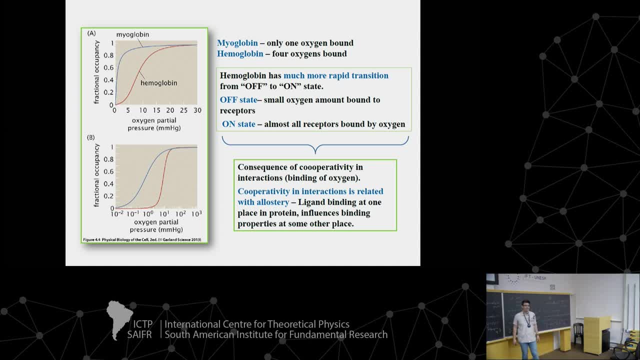 So myoglobin is sort of similar, in a sense, to hemoglobin, But what happens is that myoglobin binds only one oxygen molecule. So in hemoglobin you have four oxygen molecules which are being bound, and they are bound cooperatively, which means one molecule binds and then the other three will be included. 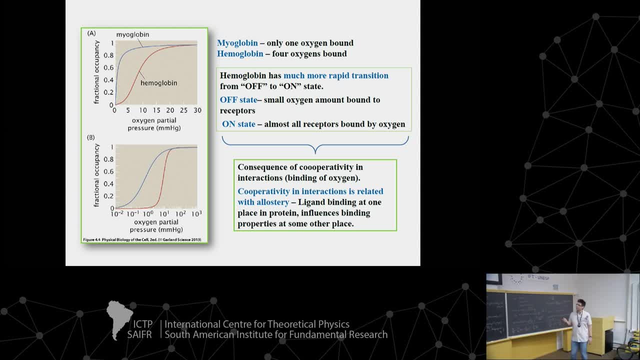 In myoglobin. it is only one molecule. And now you can also view this, this binding curve, This binding curve on a logarithmic scale. So just compare this red curve corresponding to hemoglobin, that is, to cooperative binding, And look at this blue curve. 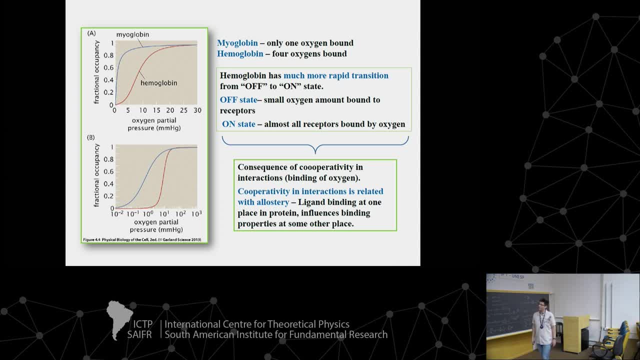 This is myoglobin, where you don't have cooperativity. But what would you say? What is the main difference between these two curves, the red one and the blue one? How would you describe it? OK, shall I try. So you see, in hemoglobin. so first there is nothing. 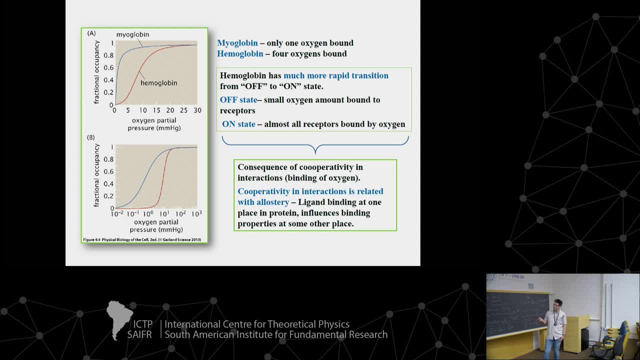 So the occupancy is zero, But then you have very rapid transition from this zero to one meaning you have very rapid transition from off state to on state, And this is actually the basic property of cooperativity: Wherever you have cooperativity, you have this switch-like behavior meaning system. 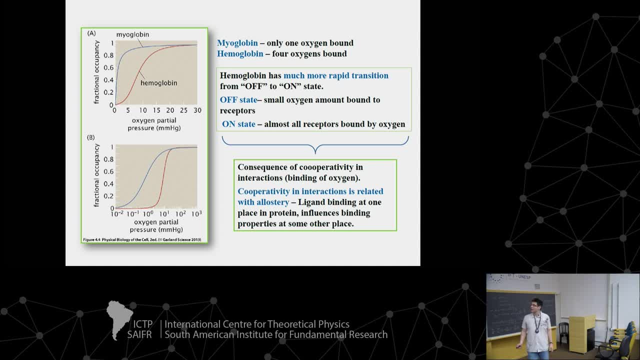 going from off, from zero basically to one, And if you compare it with myoglobin, here you do not have this switch-like behavior, here You have very gradual transition from zero to one. And now you can imagine, for example, this red thing being, for example, a toxic molecule in a cell. 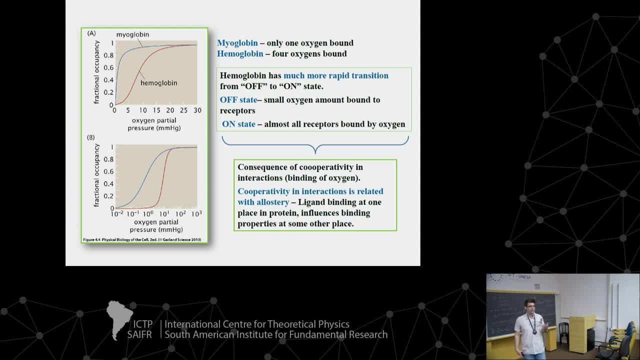 So if you have a toxic molecule, it can defend your cell from foreign DNA invasion, For example. this is what is exactly what is being done by immune systems, But then, of course, with toxic molecule, you can have autoimmunity as well. 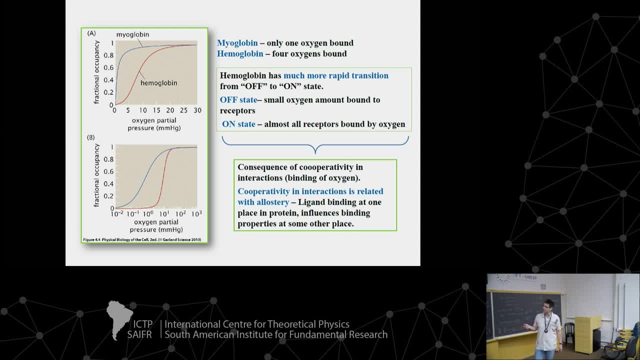 It can attack its own cell. So then in this case, this red curve, it becomes Question: No, I mean still, no, still, the red curve is steeper here. So I mean: well, I'll show the equation on this. 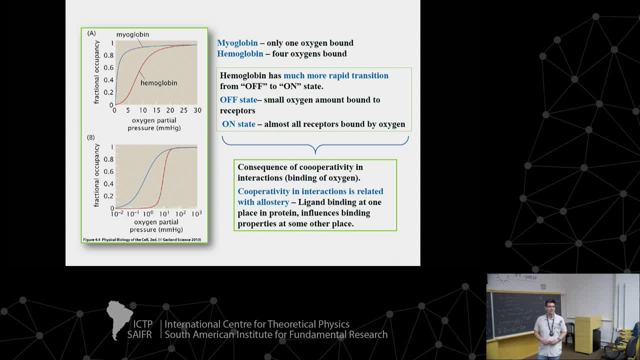 So it will be. it's Hill's curve, So evidently it is. Why do you have to tell the person to look at the scale of death to be able to explain that? Well it's. You will see the equation in a moment. 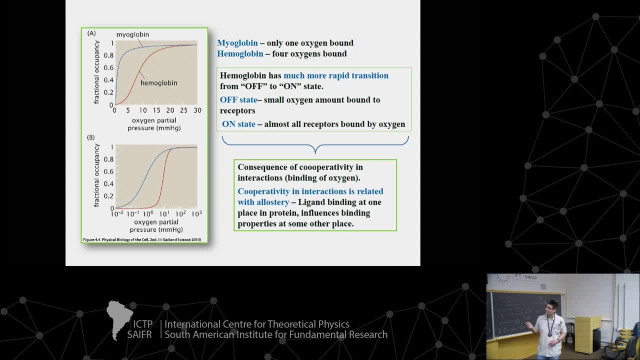 but it's just, you can see it more clearly from the red curve. But I mean, it's just, it makes the much rapid transition. So it's The Hill curve. So basically you can get it directly from here, right? 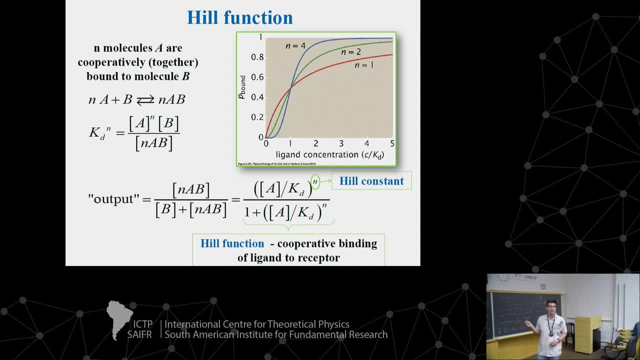 So in the case of hemoglobin it's four here right. In the case of myoglobin it's one. So evidently you know you have much faster transition from off to on state. It's just that you can see it more clearly on the logarithmic scale. 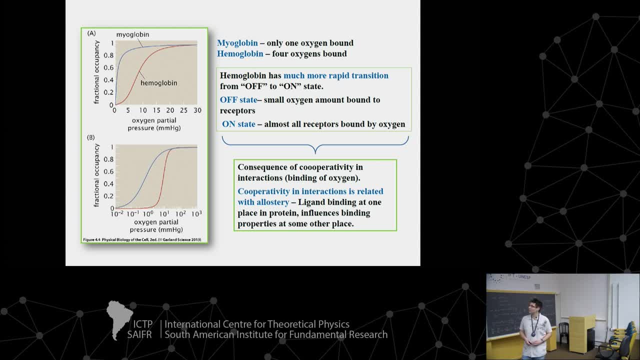 OK, Right. So what they mentioned is that: well, if you imagine that this is a toxic molecule, so it can be very useful to have it off first, right to have it at zero. In this way, you are giving time for antidote to protect. 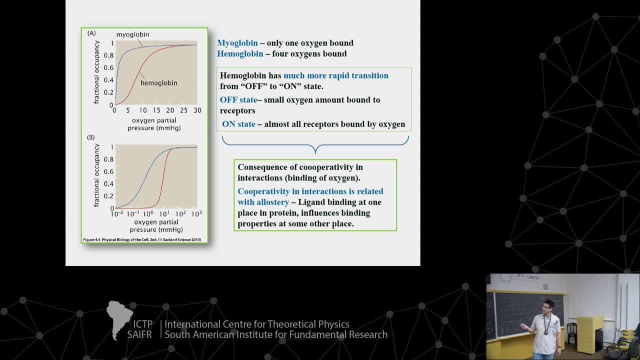 the whole cell so that you do not have autoimmunity. But then, as soon as this happens, as soon as you have protected the whole cell, you want your system to be turned on as soon as possible so that the cell can be protected. 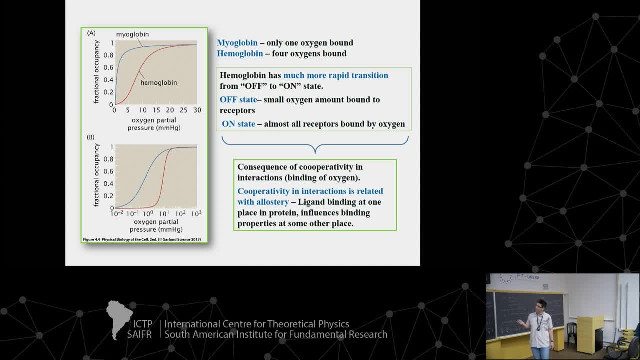 And this is this rapid transition of the system from off to on state, And this is actually the trademark of cooperativity. Wherever you have cooperativity present of the system, you will have this switch-like behavior, rapid transition, basically from zero to one. 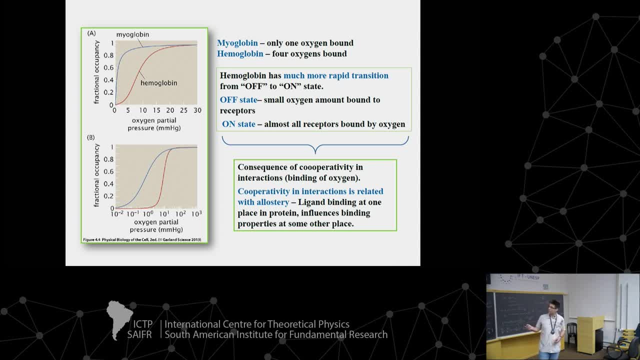 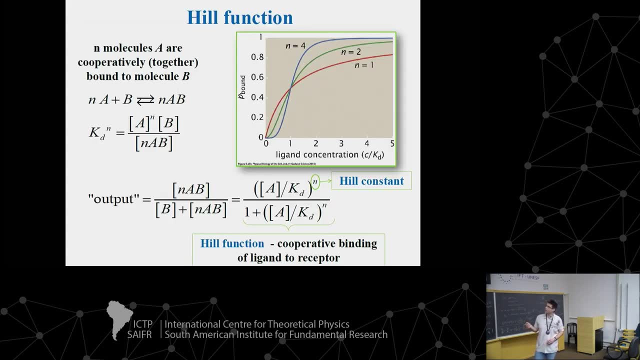 And the larger the cooperativity will be, the more rapid this transition will happen, And let me make this sort of more formal. So B is our receptor again, And then we have N molecules of your ligand which is being bound to your receptor. 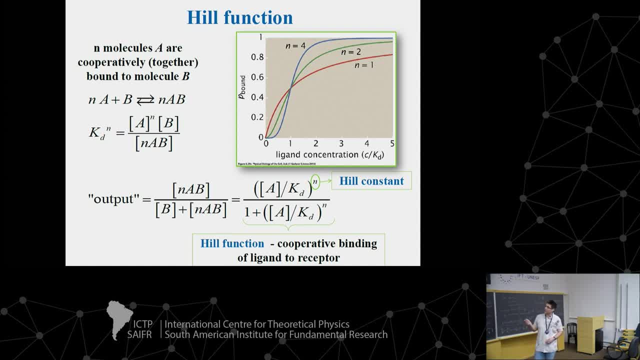 And you have a complex here. Again, you can write in equilibrium, you can write the dissociation constant for this reaction. Now, the only change is that now you have A to the power of N here, because you again multiply concentrations of the left hand side. 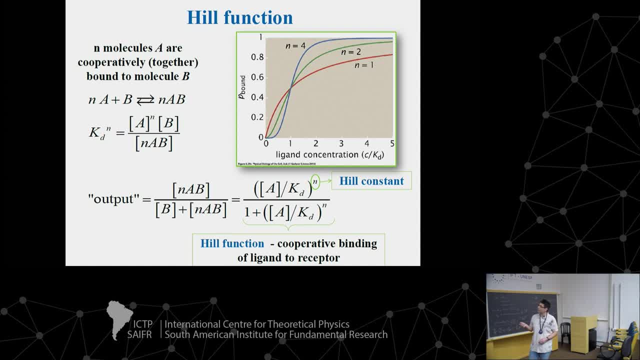 And then, if you do the same thing, so output is our fractional occupancy And then our input is our ligand concentration, You get this input-to-output relationship. The crucial difference is that you have a Hill constant here. So this is this power N. 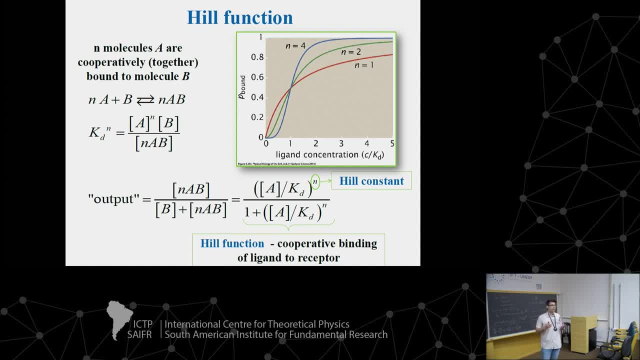 And this Hill constant is evidently related with cooperativity. More, if the larger number of molecules comes together to bind, the Hill constant will be large. And then if you plot it so now this is not logarithmic scale, so I think you can see it clearly here. 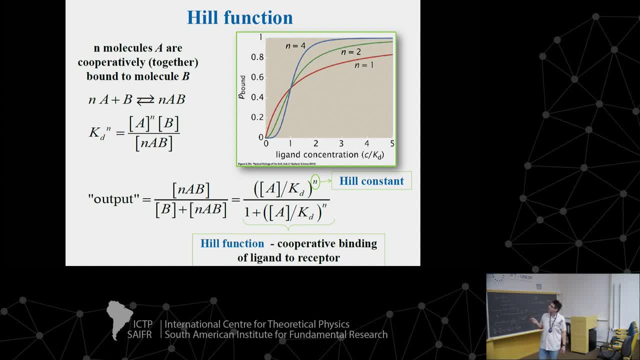 So if you plot it, this Hill curve as you increase the power of N. so you see, here for N equals to one, you have gradual transition from off to on state. then it's more switch-like when you go to N equals to two. 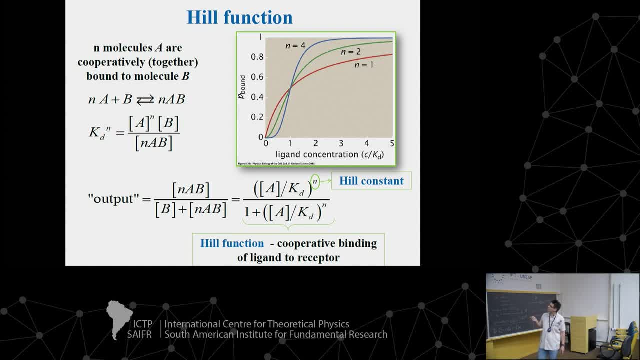 But then, for example, for N equals to four. you have very switch-like behavior, so it goes from zero and then rapidly goes to one. OK, And so, and evidently, the larger cooperativity you have, the more your system will be non-linear. 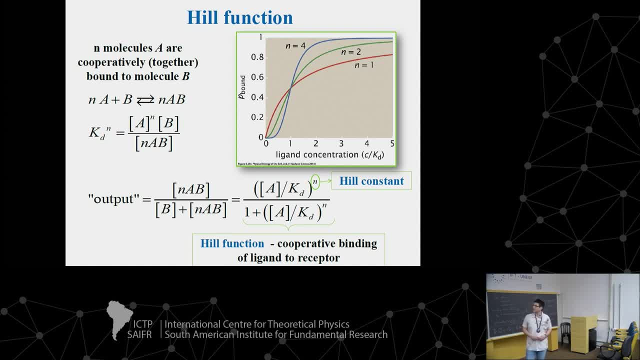 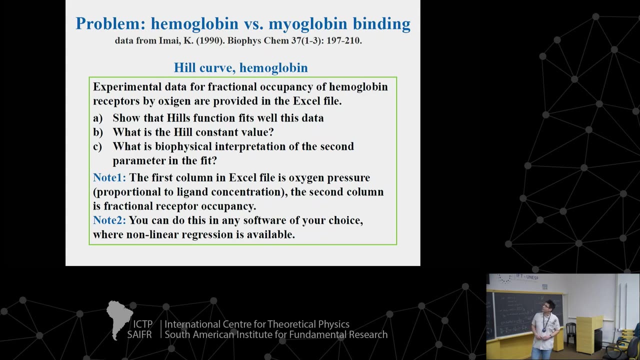 And actually with this I will conclude this part. So I hope I made the point that even at the most basic level. so if you have even single molecules interacting with each other, systems are, so to say, inherently non-linear. OK, and then here is a problem. 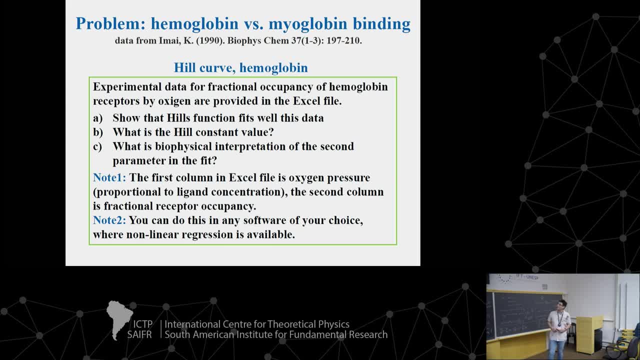 which is directly related with this hemoglobin to myoglobin data. So the data are real, experimental data, They come from this paper. So the problem, what I would like you to do, is the following: So take this data and then, just so, the data is in the form of the Excel file- 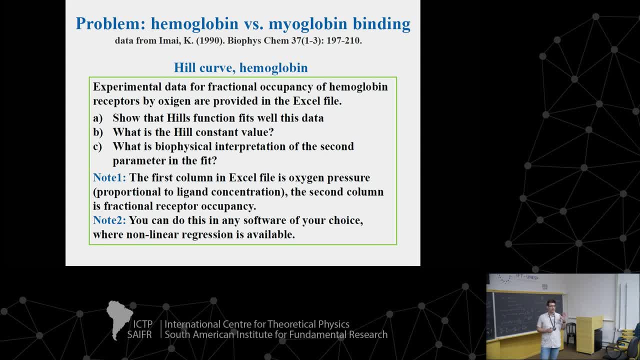 So in one column you have oxygen pressure, meaning concentration of your ligand, and then in the other column you have fractional occupancy. So I want you to try to fit this Hill curve to the hemoglobin data And you will get. from this fit, you will get two coefficients. 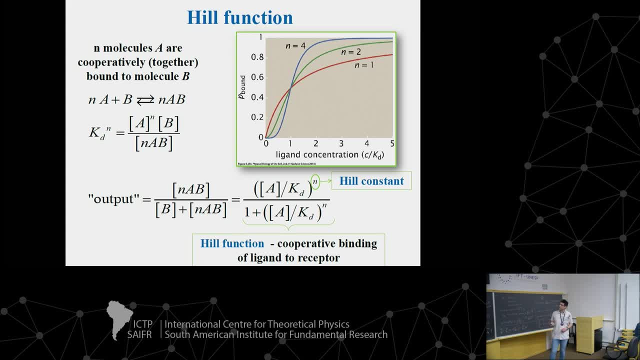 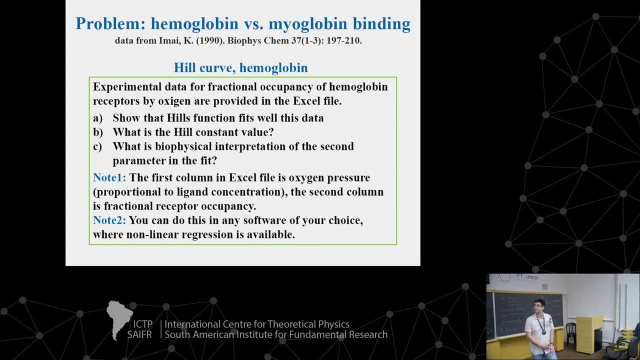 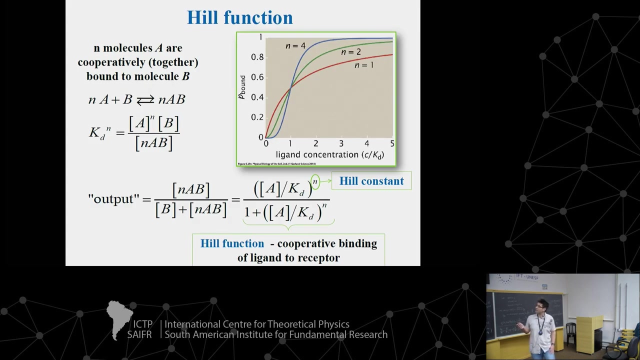 One is n, this Hill constant, and the other is this dissociation constant. So this is one of the questions in the problem. So for hemoglobin, what value of the Hill constant you expect to get from this fit? So remember, a Hill constant is how much molecules are binding together to the receptor. 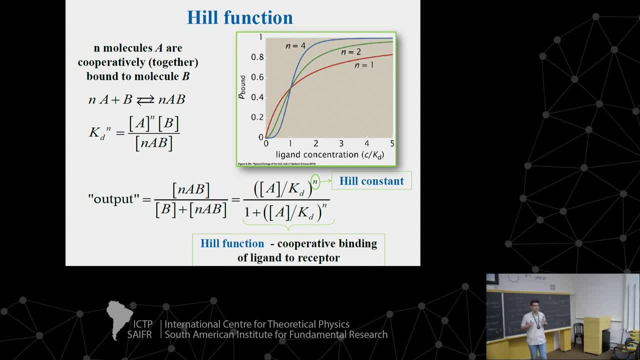 So, in the case of hemoglobin, how many molecules we expect to have to bind together? Four exactly, yeah, Yeah, so ideally it would be four, but actually I would like you to actually do the problem, so you will see, it will not be ideal. 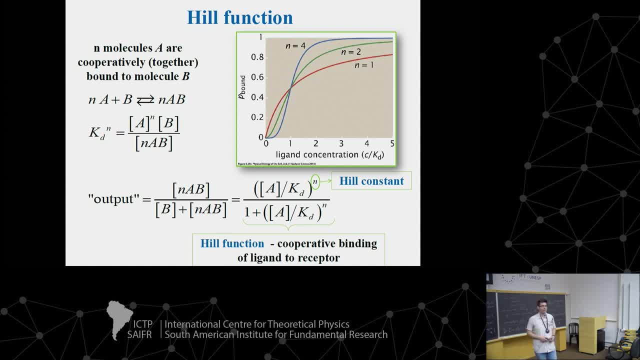 It will not be actually four, but you will see what you will get, So it will be the number which is smaller than four. Basically, this cooperativity is not ideal. When one molecule binds, you will not have always all three other molecules being bound to the receptor. 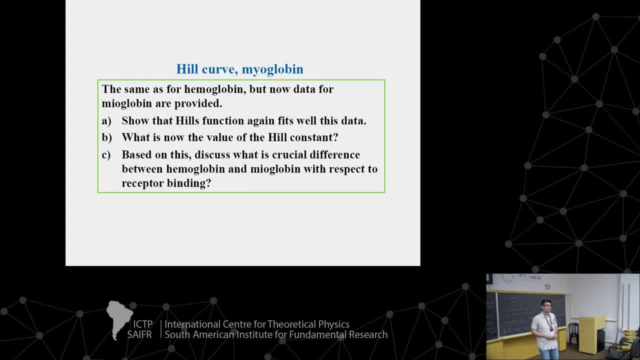 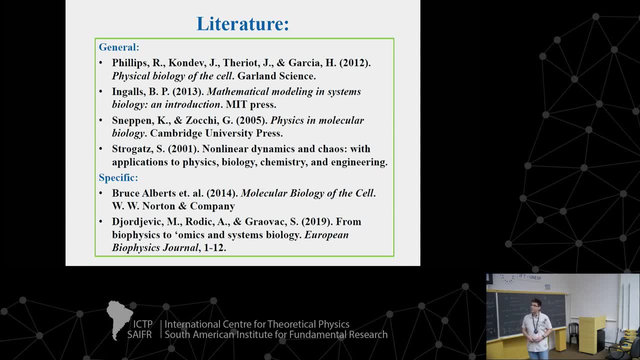 And then you should do the same thing for myoglobin as well, to compare things. OK, And now, so I have enough time to conclude with the literature. So I wanted to provide, basically, some overview of the literature which you may find useful as far as systems biology is concerned. 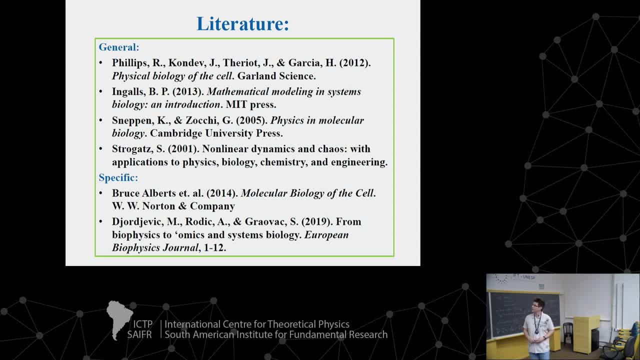 So here is the list of the general literature And here is like specific literature for this lecture. I will not come back to this general literature, but in the next lecture I will list sort of specific things for each lecture. But now let me start with specifically the truth. 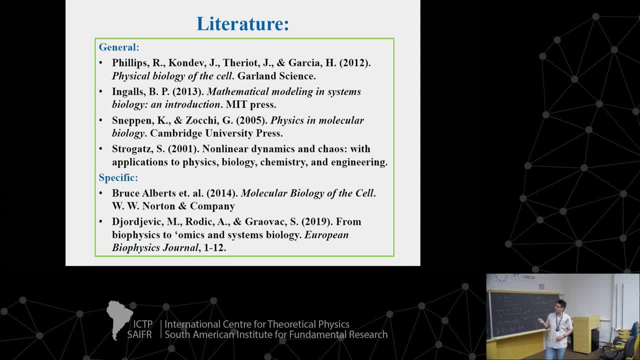 So this is one classical textbook in molecular biology. It is written by Alberts and other authors, So basically by a group of people from UCSF University of California, San Francisco, And it is really basically a very nice introduction to molecular biology. 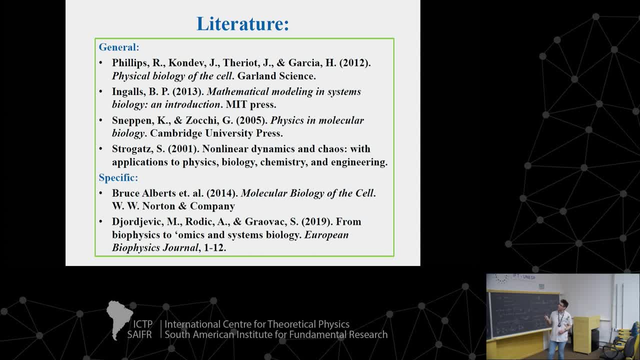 And I'm also mentioning this because of this first reference here. So this first reference is sort of paralogue of this molecular biology of the cell. It is called physical biology of the cell. It is very nicely written. It is also sort of a relatively long textbook. 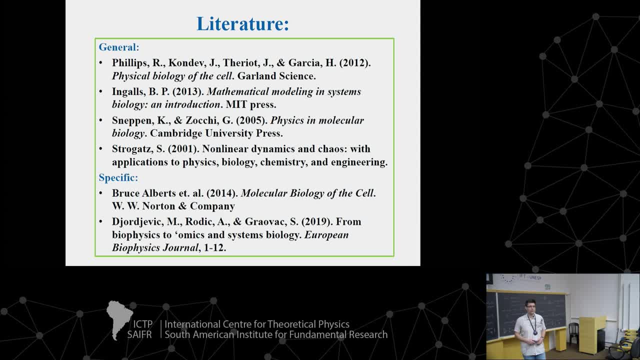 And it is basically one of the most often used textbooks as far as molecular and cellular biophysics is concerned. Actually, by chance, we have a collaboration now with one of the authors of the book. So there is this Serbian Science Foundation and we have grants with Diaspora. 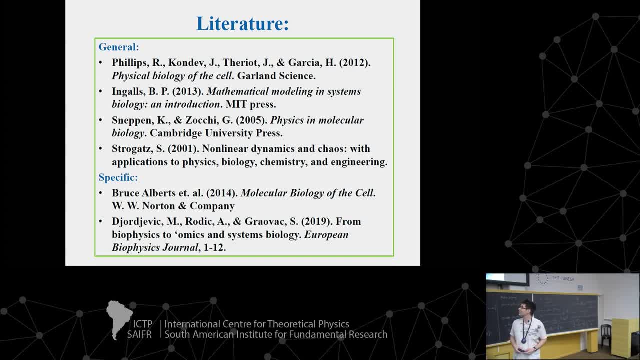 So Rianne Kondev is actually Serbian. So so we have collaboration with one of the authors of the book And then actually sort of more more brief and more, in some parts more brief and more concise version of physical biologists of the cell. is this physics in molecular biology? 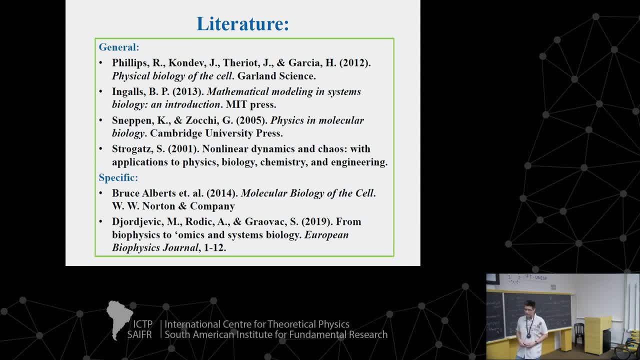 So advantage of this book is that it is more briefly written, But then on the other hand side, it is sometimes it's more, more hard and more hard to follow. Also, here you have a standard text in systems biology. Now there is perhaps some redundancy in the title here. 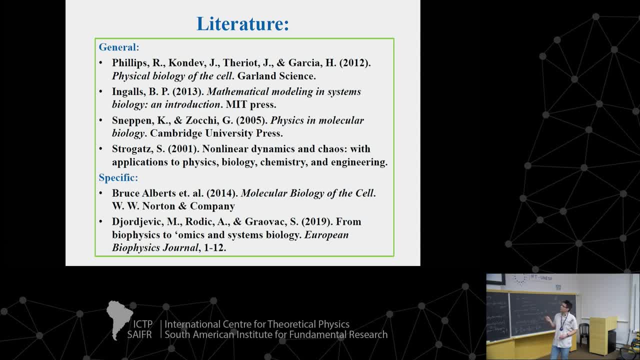 So what you see here is mathematical modeling in systems biology. So I should mention, to a large extent Systems biology today becomes essentially identical to mathematical biology of- I'm sorry- mathematical modeling of biological processes. There are also some experiments which are sort of associated with systems biology. 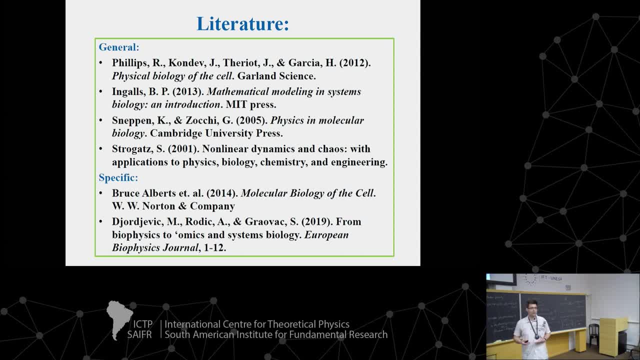 But by most what systems biology is using is just ordinary experiments that biologists will normally do, say biological lab next to you. And I should also mention it's not necessarily an introductory text. There is some Also some more advanced topics, like stochastic modeling, which are covered. 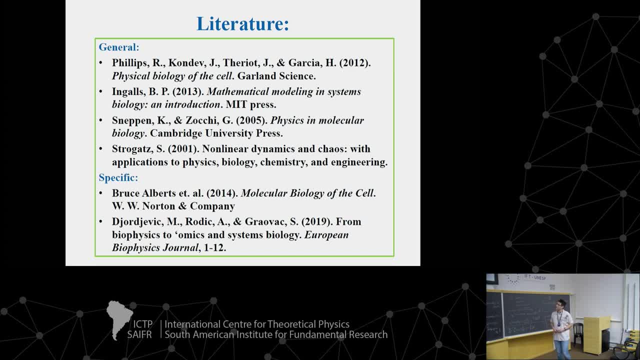 in this text. so it is more like intermediate text And also I was not well, it was not that relevant for this lecture, but it will be relevant for the next two working sessions. So this is standard textbook in nonlinear dynamics. It was written, I think, back back in 1980s. 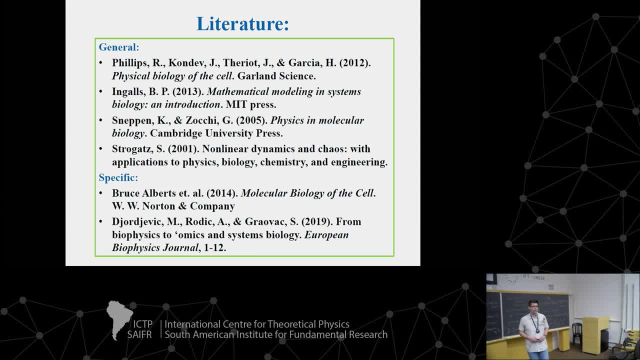 But with many minor changes in the textbook, it is still perhaps one of the most clear and one of the most used introduction to nonlinear dynamics And also as a last reference. so some of this general discussion of of why quantitative modeling may be useful in biology is also in this, in this review. 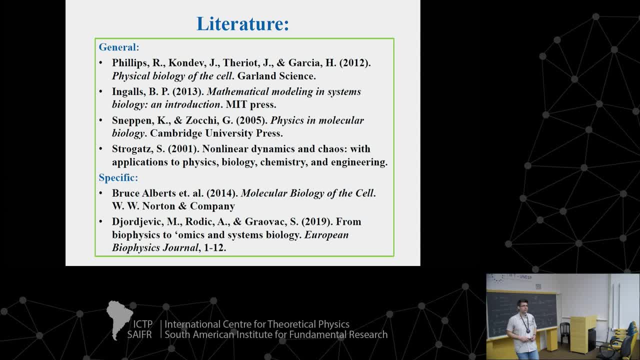 You review papers of ours, So what I should mention, in this folder that you have, you will find the lecture itself, You will find this data for the problem And then, finally, you will find, you will find this review paper as well, Of course. I mean, I was not including the textbooks. 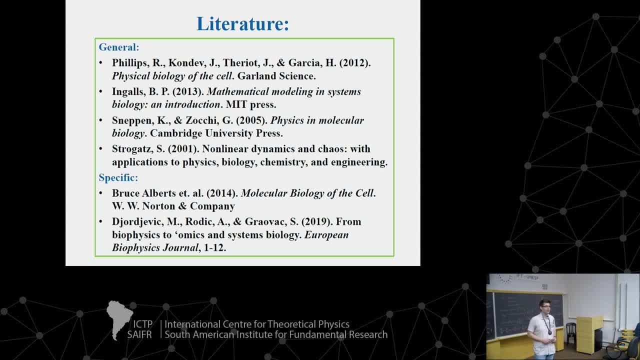 You can find them in most of the libraries, So OK, OK, so thank you very much. It's a comment about how close biology has come to physics, To a real theory predicting and verifying In physics. Newton's theory of gravitation is such a theory. 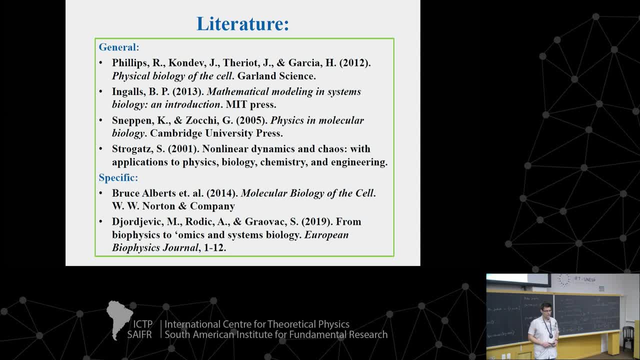 You can predict the positions of planets and so forth, with restrictions, of course. it may have sensitivity to initial conditions. You can even get to chaos. However, in biology, what you have is a self-organizing, open, evolving, dynamical system. 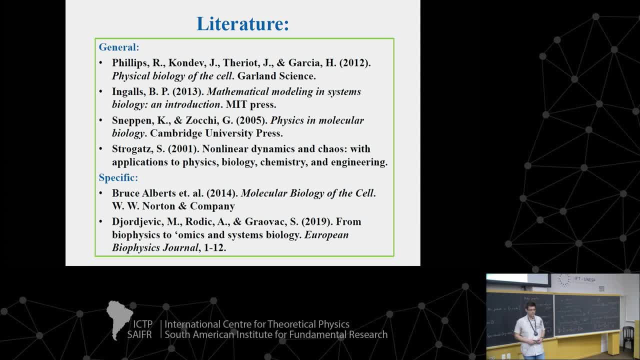 And there is no mathematics that can handle that. so far, That's my comment, Right? Well, yes, so actually we were having a discussion like this. I think it was yesterday, So I think someone was asking: for example, can you take the entire cell? 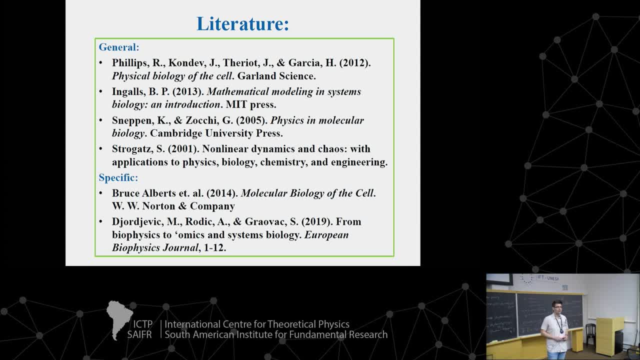 and then can you make the model of the entire cell, And then- well, people are doing this nowadays as well- For example, for a minimal cell you have complete models of sort of minimal cell and things like that. But then sort of I mean, if you do things like that, 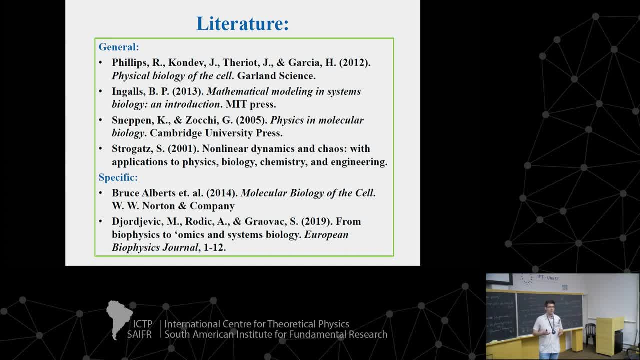 if your model becomes as detailed as the entire system, then what is the point of the model? Then you should better be doing experiments. So what I would say is that in systems biology, the main purpose is actually to catch the main properties of your system. 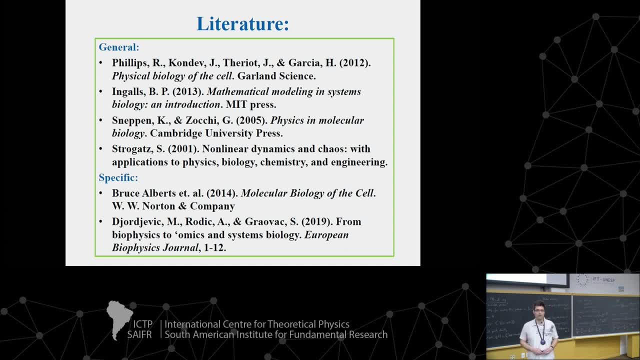 the properties which are most important for the phenomena that you want to describe. So it's not, I think, a goal in the sense of Newtonian mechanics, to take the entire cell in its complexity and to entirely predict its behavior, but actually to extract what would be the most important for the system. 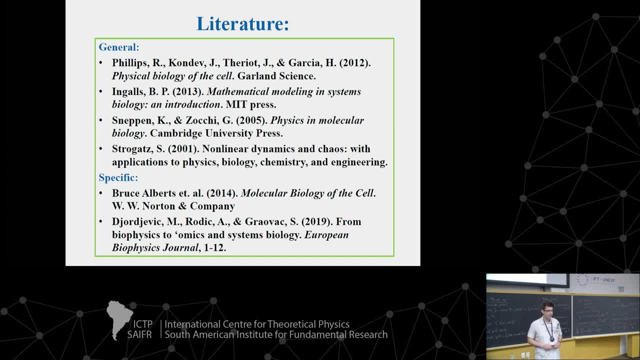 And what can explain the phenomena that you're looking at? Yeah, but what mathematics cannot do is deal with a system such that the evolution of the system changes the structure of the system. That's the crucial point, Right? but it depends on what time scales you're looking at. 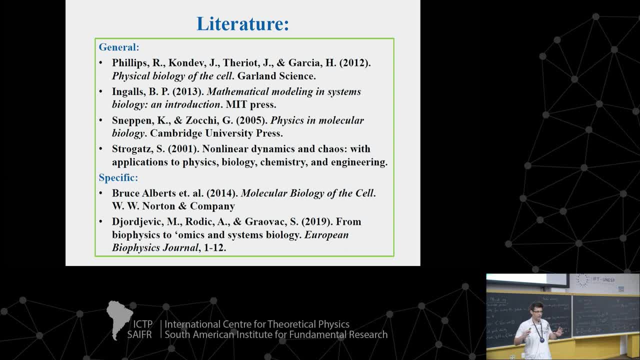 So if you're looking at evolution, so it is one long time scale. So it is how bacteria is changing, how it is acquiring genes, how they become resistant and so on. But say that you want to model your system as it is at a given time, right? 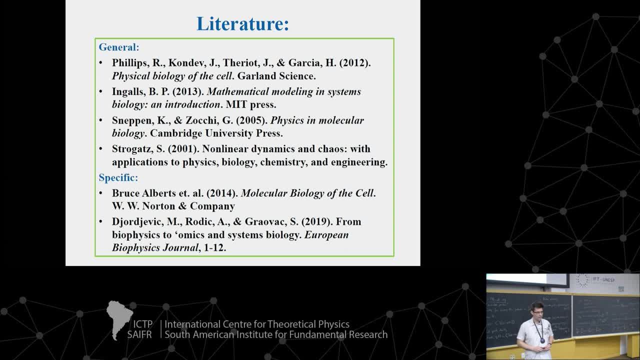 But how some organisms will grow as a living system. Right, but just what I want to say, it's sort of two separate things. One is how they evolve, how they change, But the other thing is describing the system at a given. you know, as it is now. 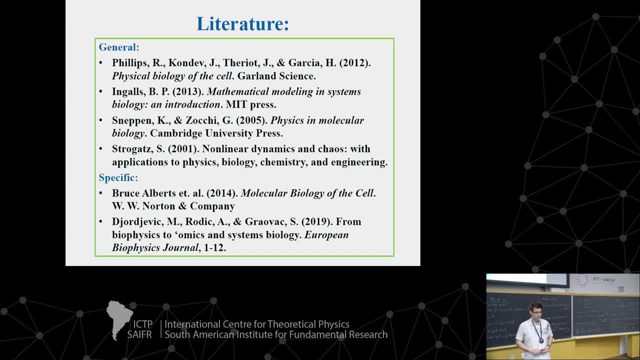 for example, equally as You can use statistics, I mean kinetic theory of gases is a model using statistics and so forth that needs prediction of properties of gases, But that's not really a theoretical, I mean a mathematical theory. 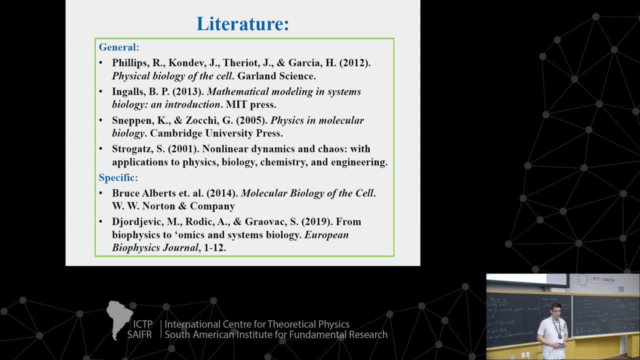 That's the point that I'm trying to make, Right? okay, That's a valid comment and it's probably tragic, Okay, So, uh-huh, I'm sorry, if you can, just if you can- just a little bit louder, sorry. 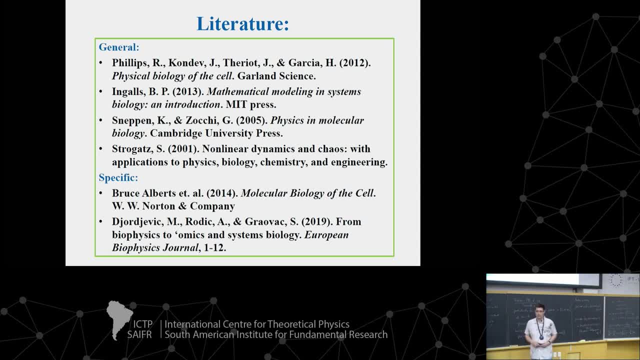 Yes, of course. So whenever you have cooperativity, you can do that So well. actually, this would be this gene network thing. for example, it can be one transcription factor, It can regulate gene B, and then B can regulate C. 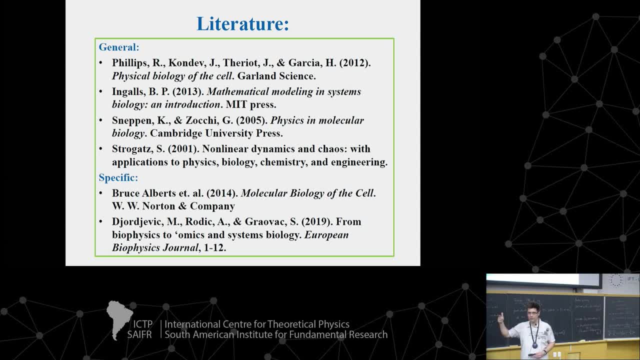 So. so essentially whenever you have cooperativity you will have Hill function essentially there. But actually there is nice mathematical weights. It will actually be in the third lecture. So you use statistical thermodynamics. It goes to basically whenever you have some conformation of molecules. 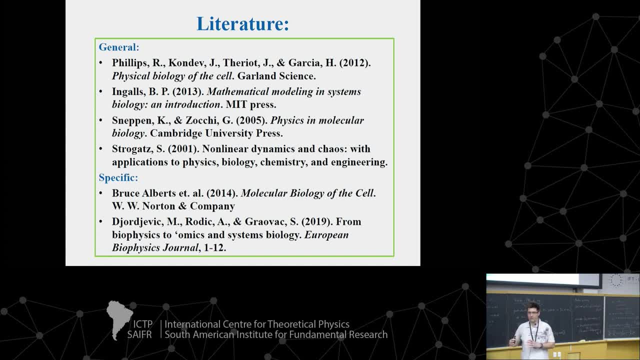 you can assign specific statistical weight to it. And then let me say that you want- sorry, then let me say that you want- to calculate probability of some configuration happening. You will, you will have your, your statistical weights of, of of you know. 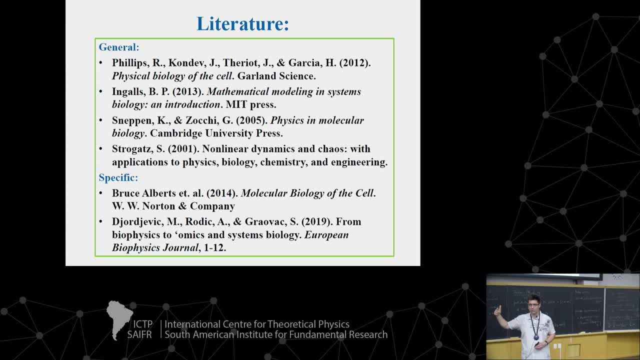 basically the configuration that you want, for example, descriptionally active configuration, divided by your partition functions, meaning by statistical weights of the entire configuration. So so in this way this cooperativity or Hill function will naturally happen. But what I'm trying to say you have very 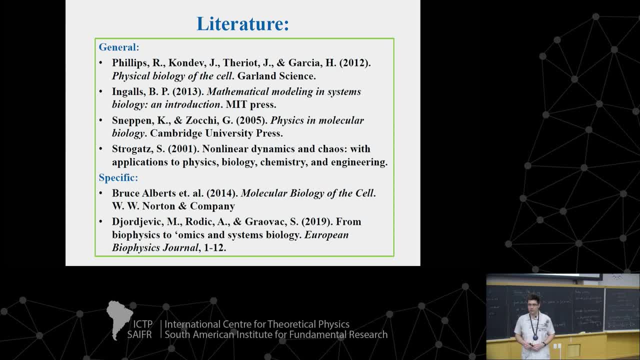 sort of way in which you can, you can calculate these things, But but yes, so whenever you have cooperativity, this, this N factor will come up, Uh-huh. So, whenever you go back to the main, my global data, 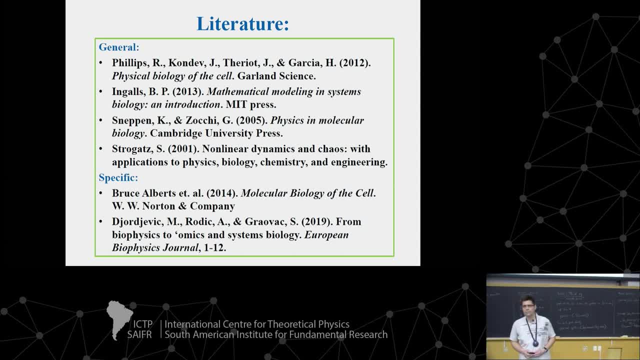 the way I understand is, the thing you're looking for is that kind of threshold. I'm sorry, Threshold. yes, You have some threshold, you know that concentration. then you have no binding and all of that. you have pretty much like pretty quick binding. 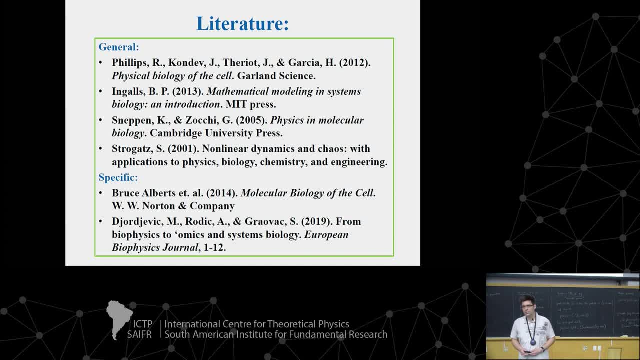 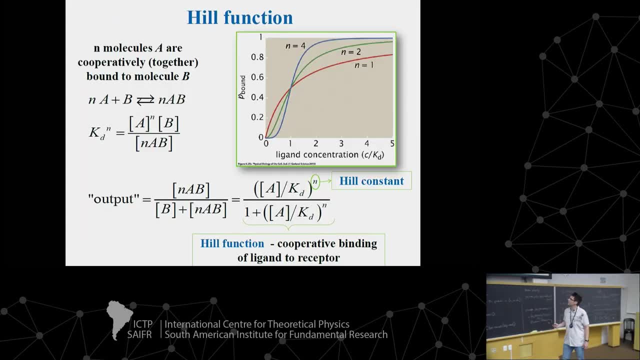 But then if you look at the mind-loving there's necessarily, you know, right, if you look at the data like that's the way I'm understanding it. Yeah, I'm sorry. Yeah, So so perhaps they didn't explain it to you. 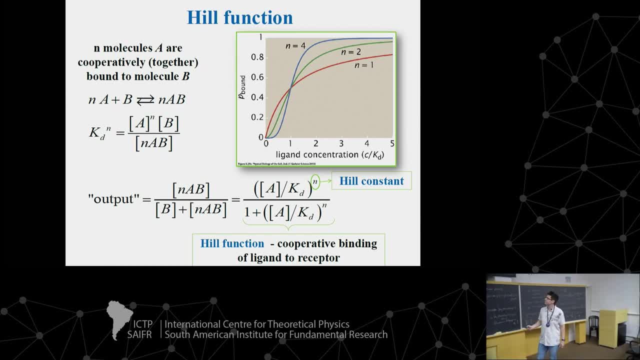 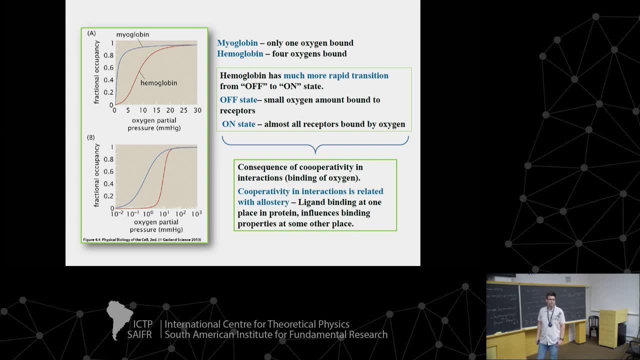 Yeah, maybe one before this, one before this? Yeah, so and then. so the reason that, the way I'm understanding it, the reason that you want to show it in a log graph on the bottom one, is because so that, even if you. 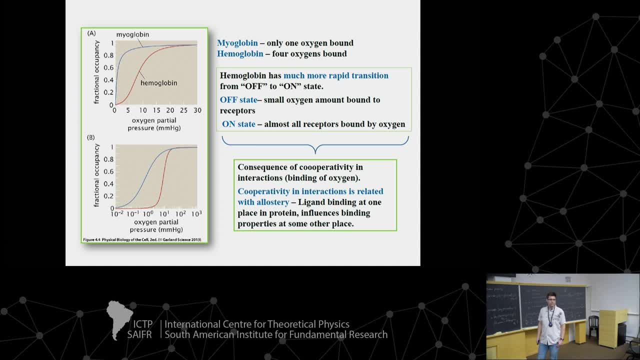 if you stretch out that point towards zero, you really don't see any threshold below which the mind-loving will have zero state. Yeah, I'm sorry, but it's really very simple. So the threshold that you are mentioning this is this: Kd. 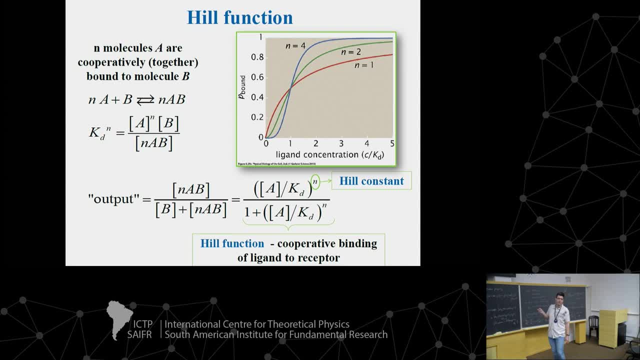 So Kd is the threshold, So Kd is concentration at which you will have half of your receptor being bound. So as you change Kd, you will change this threshold, OK. and then the other thing is n. So n will be the slope here, right, the slope of this curve.